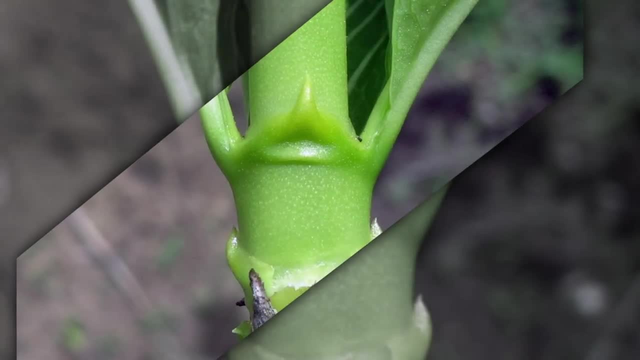 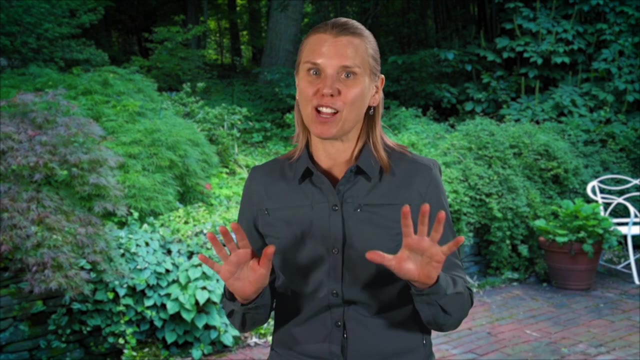 and you recognize it instantly. And that one character helps you identify an unknown plant. These terms will help you be able to talk about the parts of plants and make identifications in the field. We'll start from the ground and work our way up. 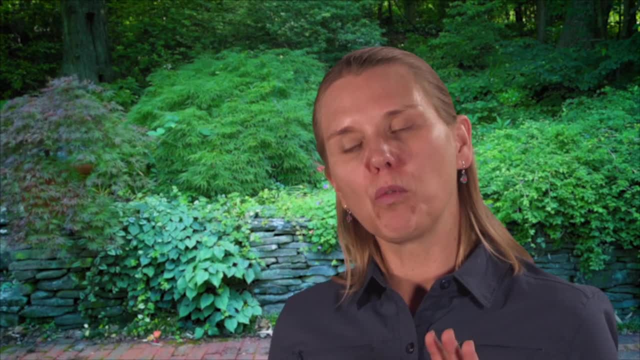 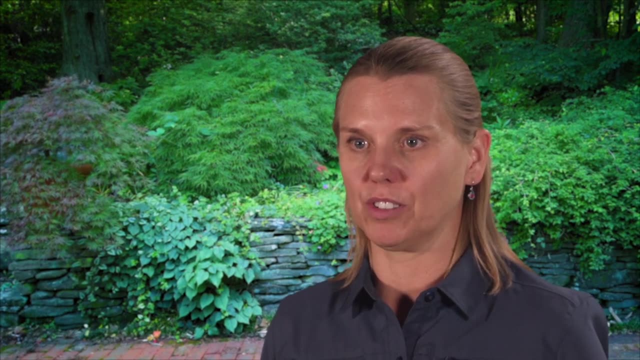 and then we'll discuss fruit types. Typically, the roots aren't used too much in identifying plants, though I do know that many grasses are indistinguishable without their roots. There are two main types of root systems. Plants can either have a taproot, 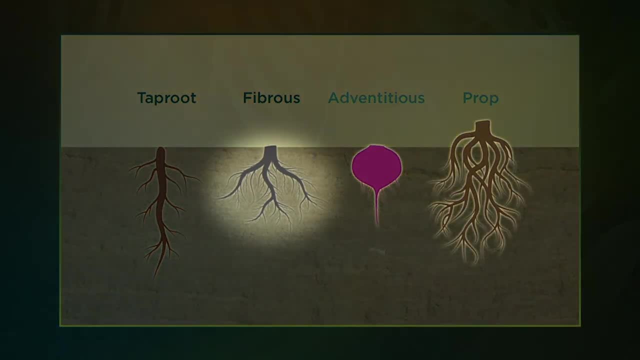 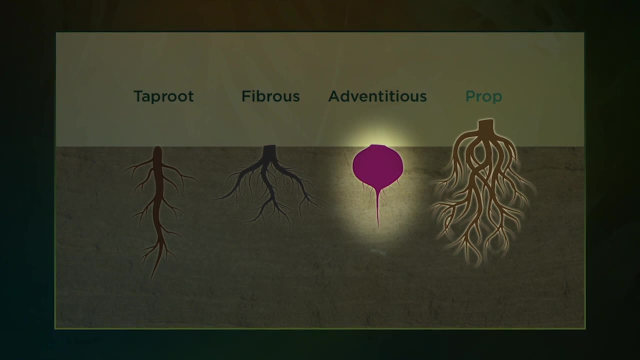 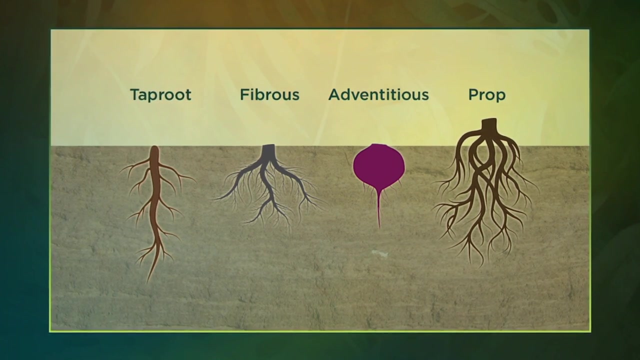 which is like a carrot or a fibrous root, but no one root is bigger than the others. Some plants can also have adventitious roots. In biology, the word adventitious means an unusual anatomical position or formed by accident. In the case of adventitious roots, 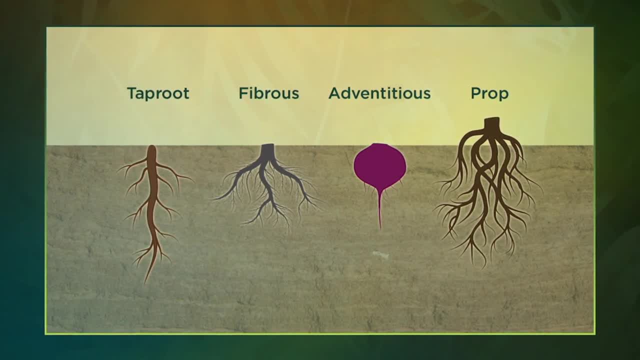 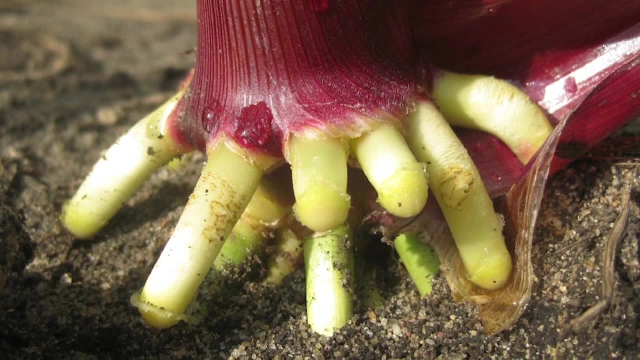 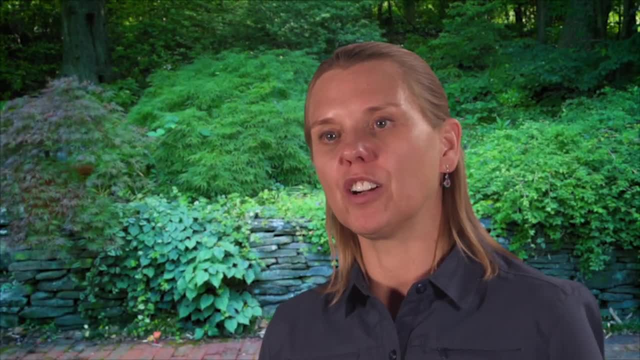 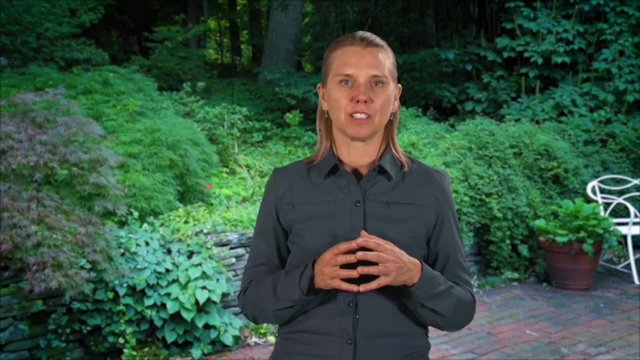 Found in mangroves. We'll discuss another important identifying traits of roots as we meet them, but for now let's know fibrous roots and taproots. Moving up the stem there is a bit more variety. Some stems are green. 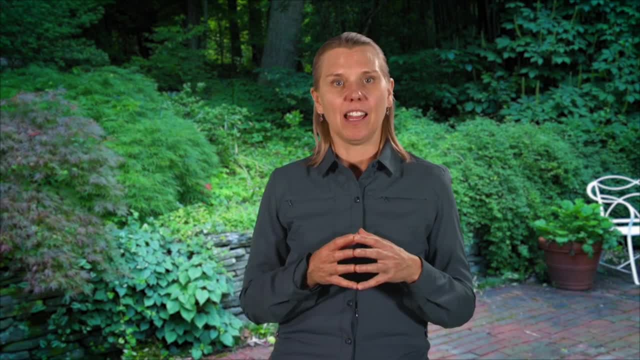 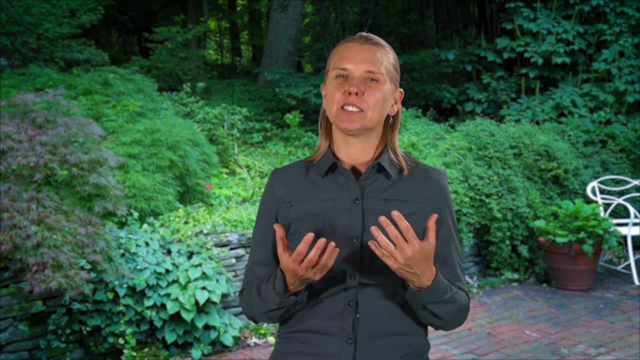 which means that those stems are photosynthesizing, and that can be an identifying trait. Mostly, though, when we discuss stems, botanists are really discussing the overall plant habit, which means growth for plants. In fact, botanists are really discussing the overall plant habit. 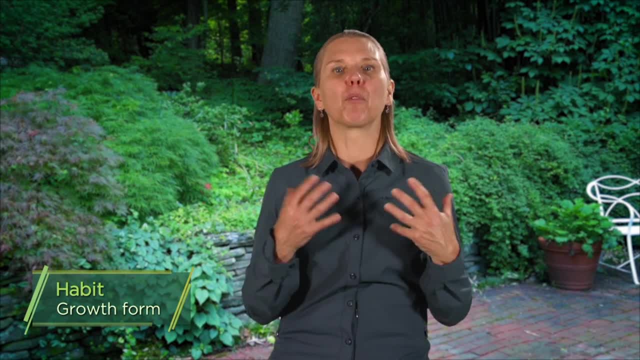 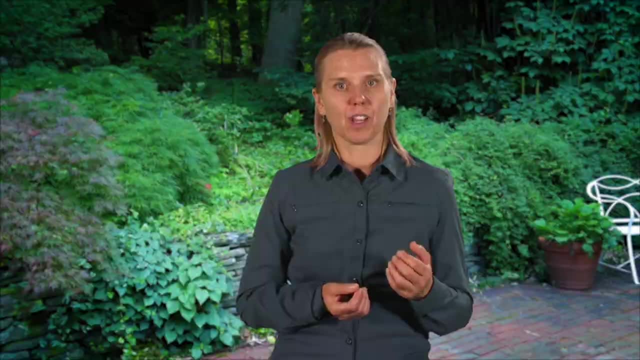 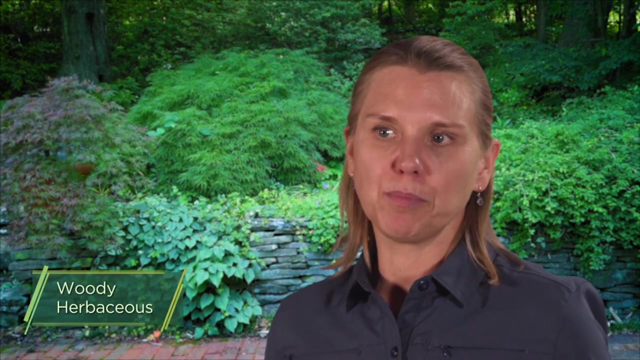 which means growth for plants. Don't confuse habit with habitat. The habit is the overall morphology of the plant and the habitat is the type of ecosystem in which the plant grows. When thinking about stems, botanists will first determine if a plant is woody or herbaceous. 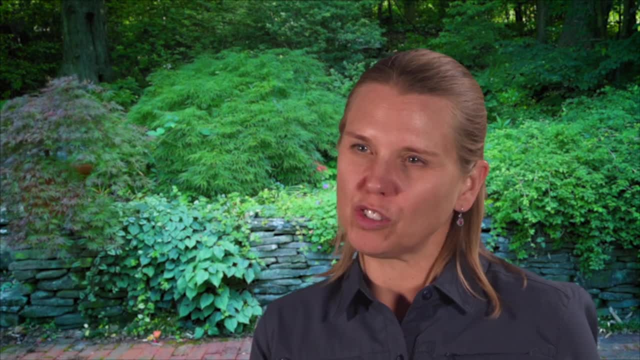 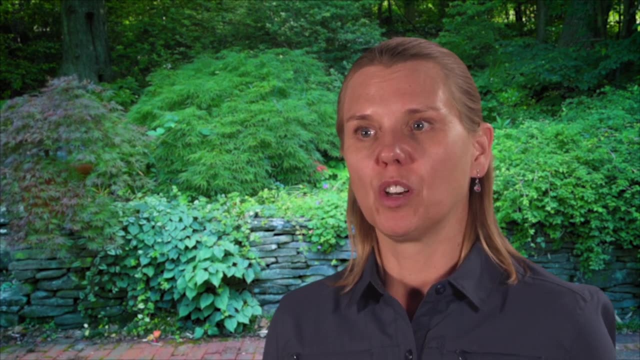 Sometimes plants might be woody at the base, so it's important to check the base when identifying this character. Herbaceous growth forms are grasses and herbs, which are also sometimes called forbs. This word forb comes from the Greek phorbae. 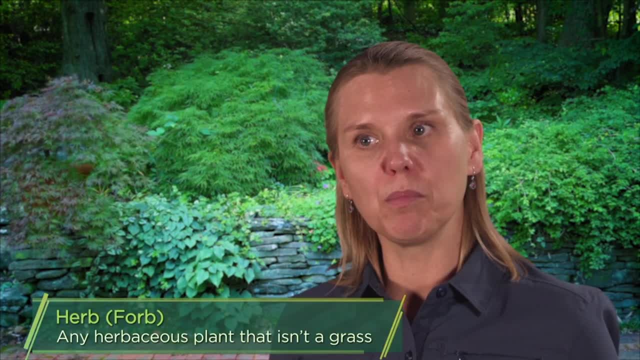 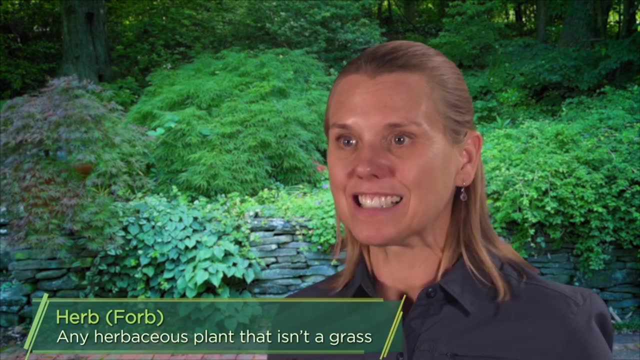 or fodder from phorbaing to feed An herb or a forb is generally any herbaceous plant that isn't a grass, so even a weed like a dandelion would be considered a forb, but so would useful fodder like alfalfa. 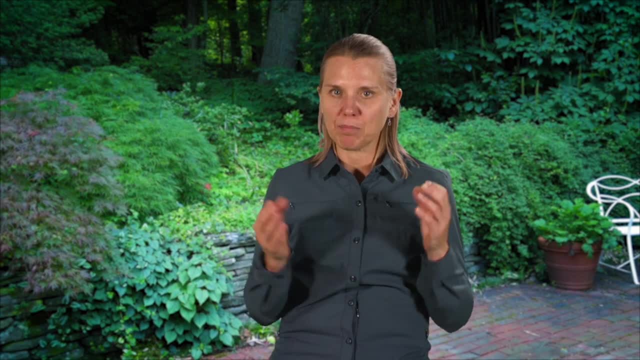 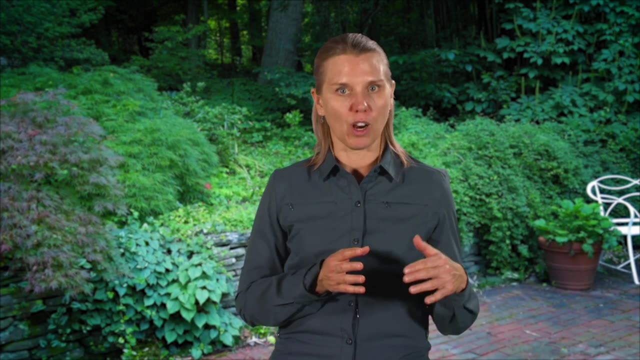 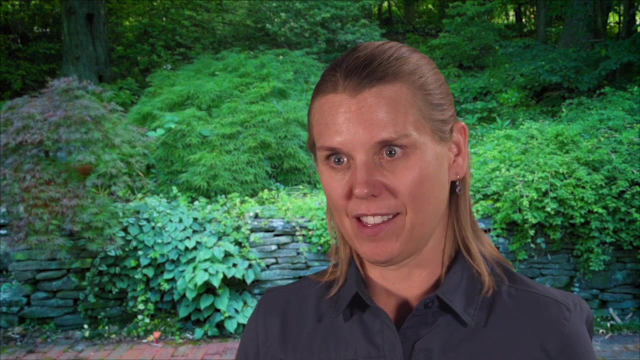 We'll learn to identify grasses in a later lecture, but for now, keep those terms in your mind. for herbaceous plants, Woody plants can include trees, shrubs and sub-shrubs, which are smaller shrubs. There are a few other words that define the overall growth. 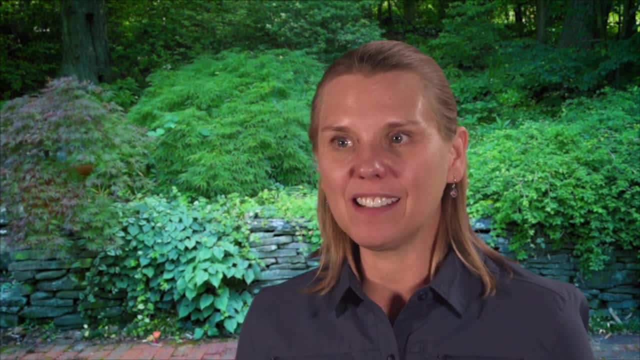 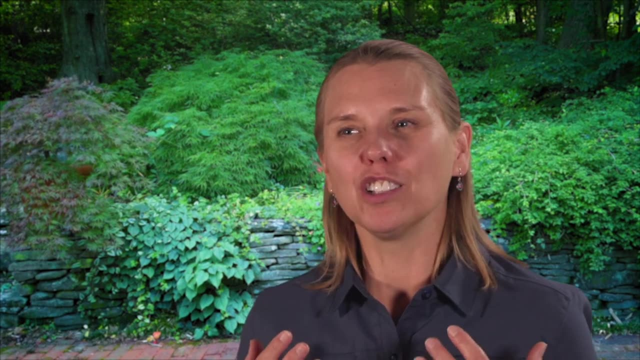 and these plants can have woody tissue or not. Again, there are other habit descriptors, but we'll meet them as we meet the families that they typify, Along with the plant's overall habit. many identification books will ask whether the plant is an annual or a perennial. 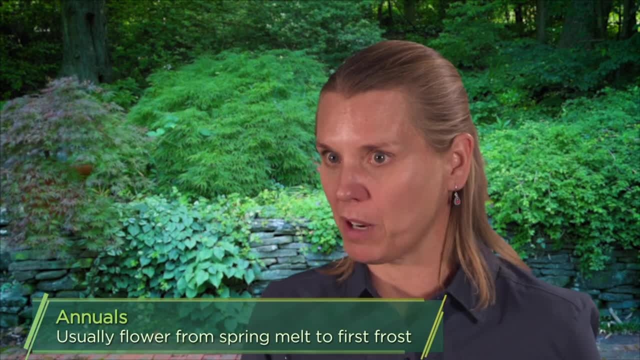 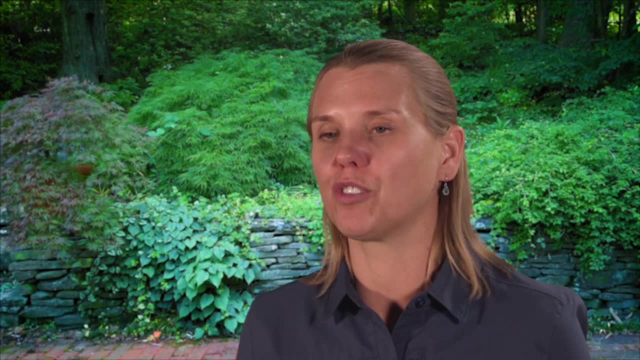 If the plant is an annual or a perennial, it will have a shorter flowering time. Annuals usually flower from spring melt to first frost, which is more true in the garden than in the field, but this is still a useful guideline. In the field, many annuals will bloom when there is adequate water. 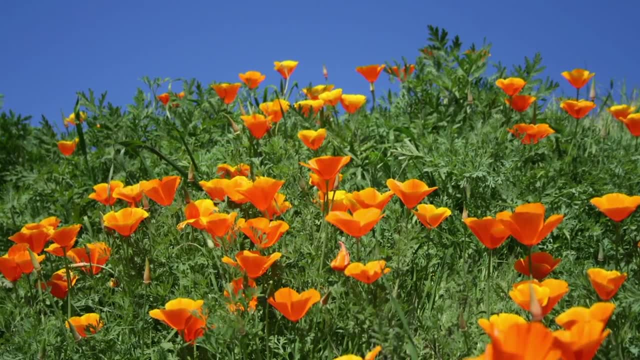 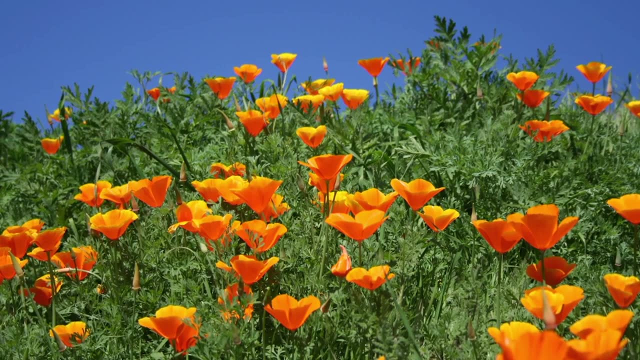 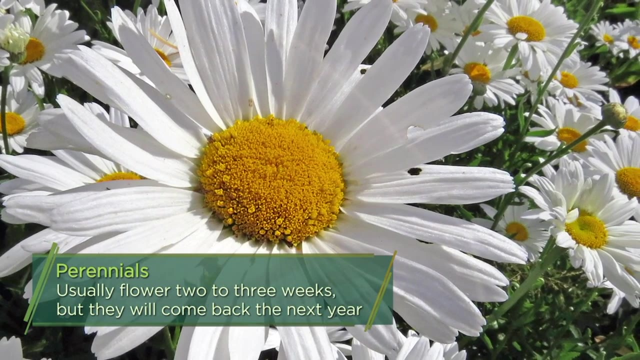 such as many desert annuals. In fact, some plants will behave like annuals in cold climates, but will be perennials in milder climates, such as poppies. Perennials will have a shorter flowering time, typically two to three weeks, but they will come back the next year. 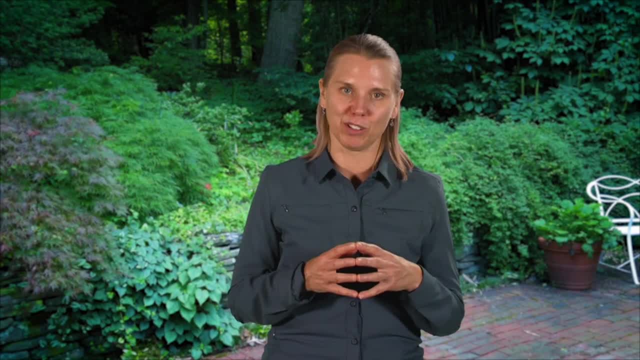 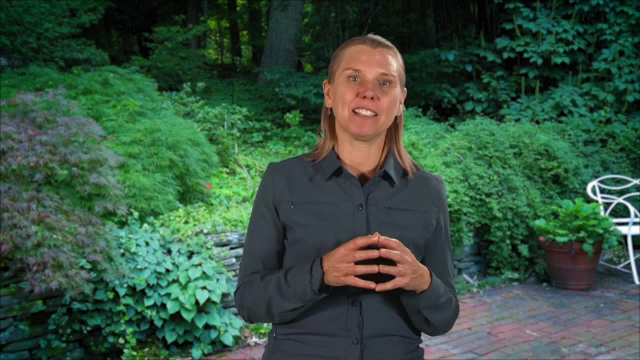 Remember that no plant lives forever, and even perennials will die In the field, anything that is woody, even at the base, is a perennial, and herbaceous plants can be either perennial or annual, and you'll have to use flowering time as a clue. 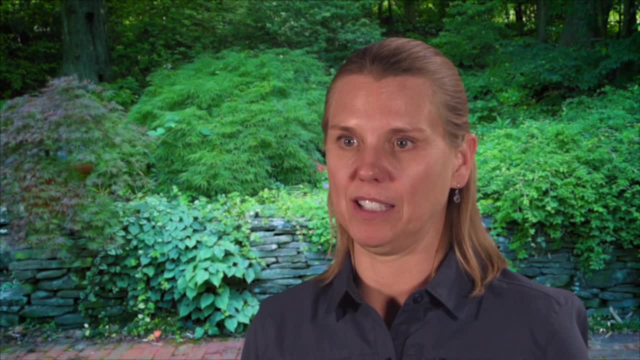 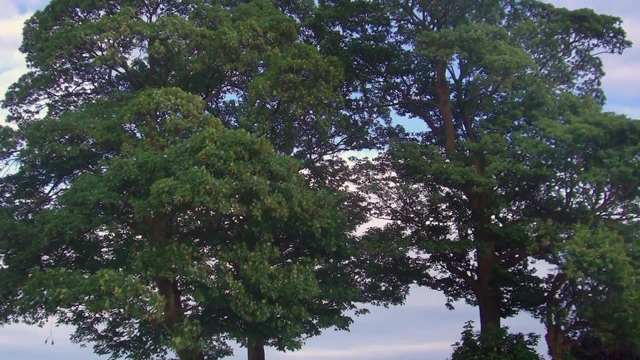 Moving up to the leaves, this is where a lot of the identification will take place. For many broad-leaved trees, the shape of the leaf and the texture of the bark are the main identification characteristics. Broad leaves means that the leaves are broad, and this is usually contrasted. 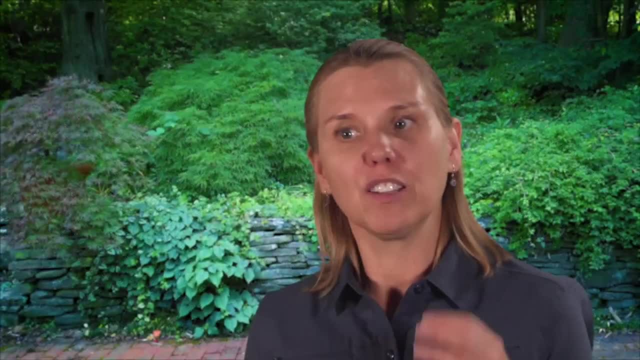 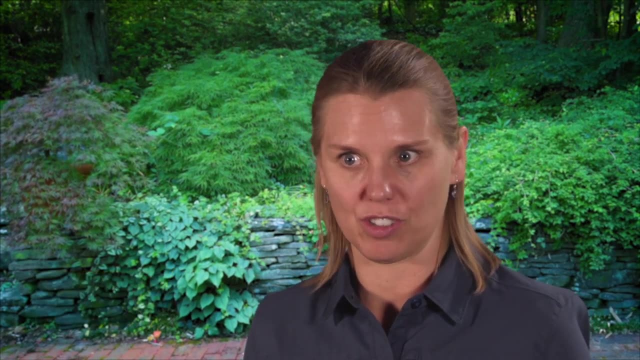 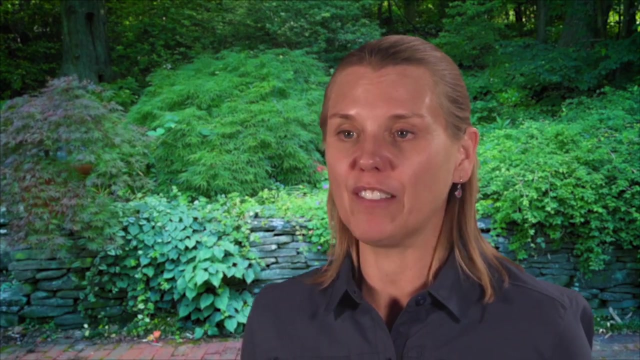 with needle-like, such as in conifers. Leaves are also classified as evergreen or deciduous. Not all conifers are evergreen- remember the larches- and not all broad-leaved trees are deciduous. In the tropics, many broad-leaved trees are evergreen. Even in North America there are some broad-leaved trees that represent evergreen trees, especially in the southern states. An example would be some species of magnolia tree and the live oaks. We won't delve into all the leaf shapes at this time. 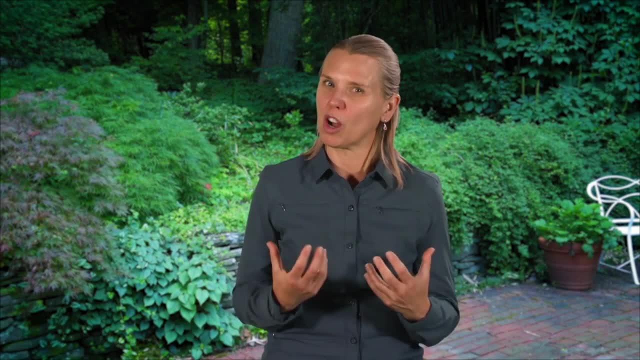 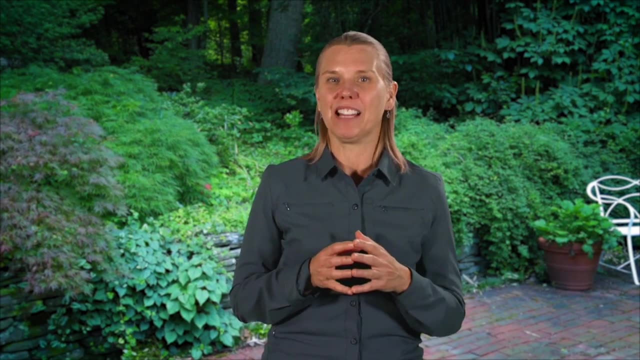 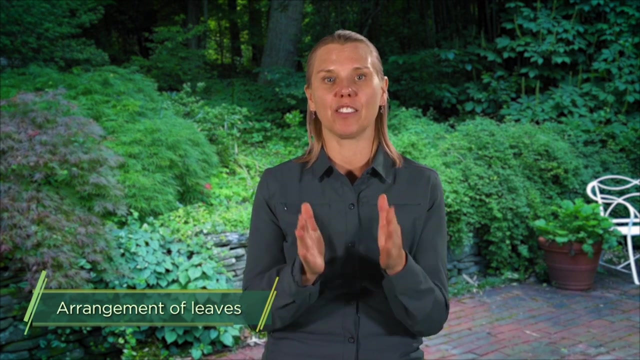 mainly because leaf shape is not a particularly strong defining characteristic for families. Leaf shape is best for defining species and we'll look at some examples in later families. What is very useful for defining families is the arrangement of leaves on the stem. The location where leaves insert into the stem is called the node. 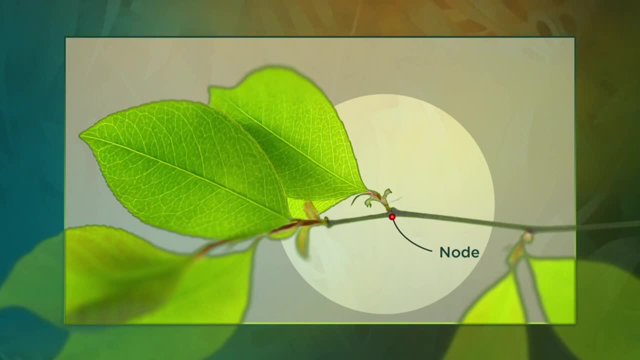 Typical leaves have a flat base and a leaf stem that connects the blade of the leaf to the main stem. This leaf stem is called the petiole. How the petiole is attached to the stem determines the leaf arrangement, and there are three. 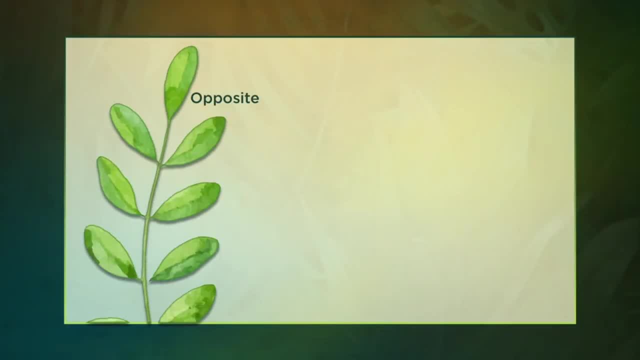 main leaf arrangements. An opposite leaf arrangement occurs where one leaf inserts directly opposite a leaf on the other side of the stem. This is in contrast to an alternate leaf arrangement where leaves- you guessed it- alternate up the stem. One way to learn plants is to memorize families with particular characteristics, such as all: 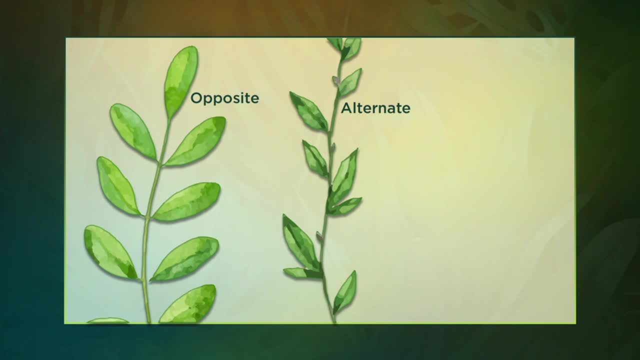 the plant families that have opposite leaves. However, there are a couple hundred plant families that could have opposite leaves, especially if you live in the tropics. Still, these are important. These are important terms to know, as they can be especially useful for determining the 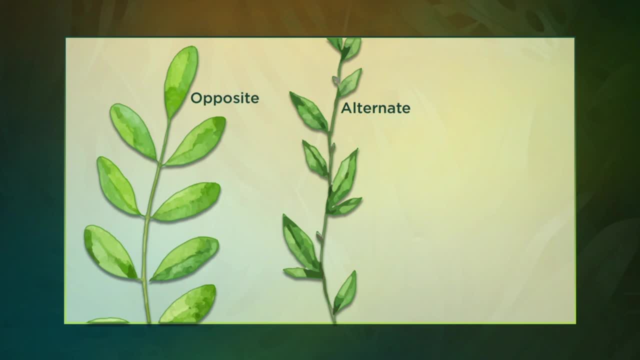 differences between two families that have similar-looking flowers. The third type of leaf arrangement is called whorled. This word sounds a lot like whorled and that's probably its derivation- the whorl of a spindle. Whorled means that the leaves are arranged in a circle around the stem. 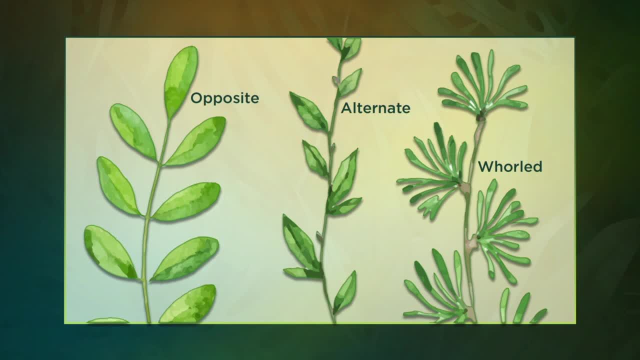 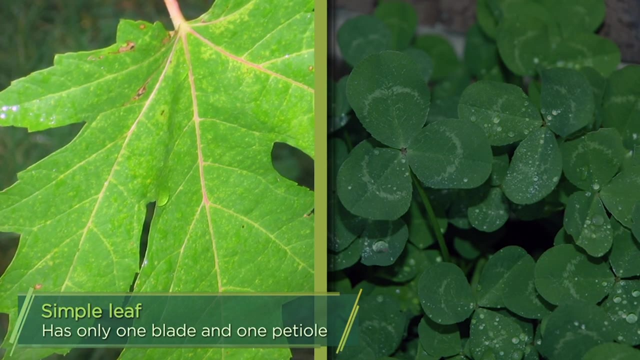 Think a whorl of whorled leaves. Sometimes it's a bit confusing to get the leaf arrangement right, and that's because what constitutes a leaf can be a bit tricky in some plants. A leaf can be simple or compound. A simple leaf has only one blade and one petiole. 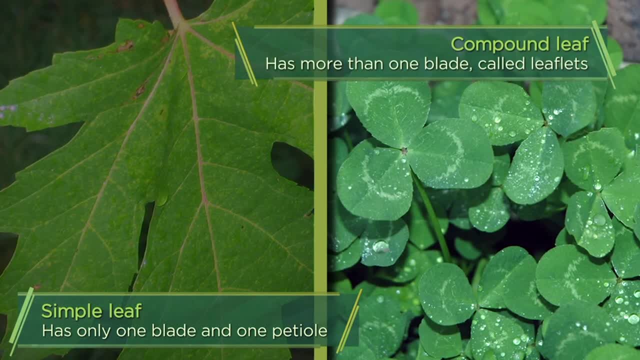 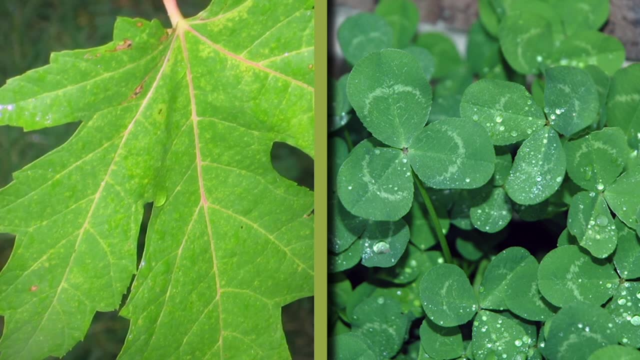 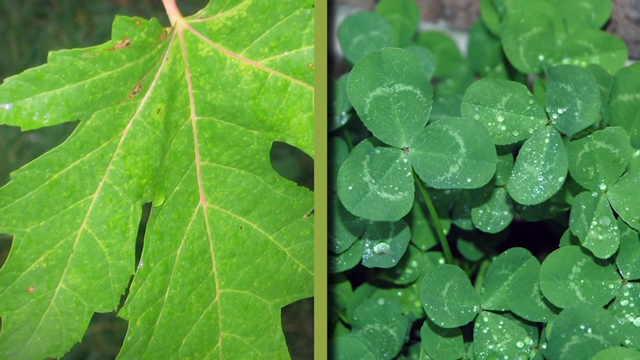 A compound leaf will have more than one blade, and so these numerous blades are called leaflets. So even though it has lobes, the maple tree is still one blade. OK, Let's see, has three leaflets, so it is a compound leaf. 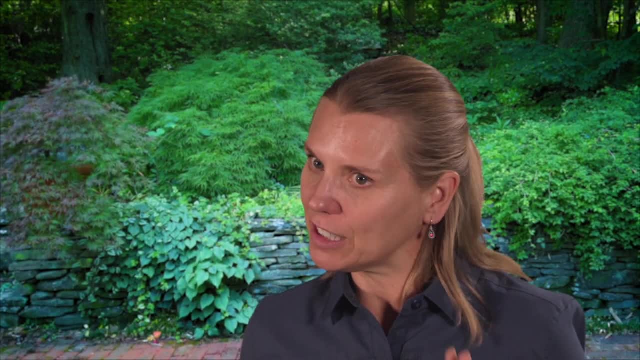 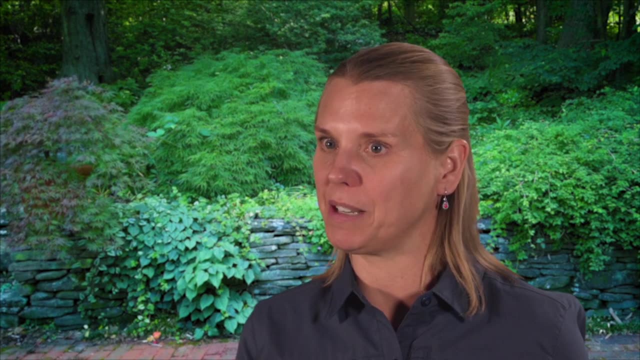 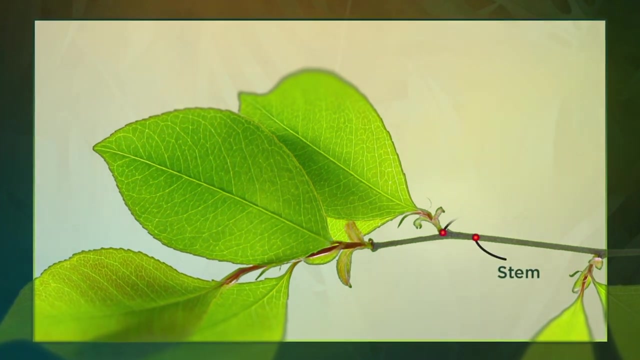 Although there may appear to be more than one petiole, there is only one, And in the junction between the petiole and the main stem can be found the key to determining if a blade is a leaf or a leaflet. When you look in the axle, which is a fancy term for the space, 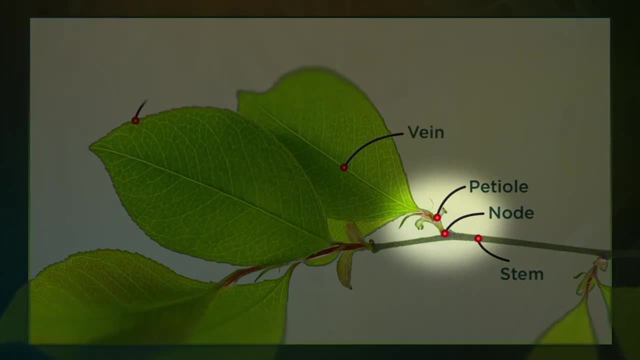 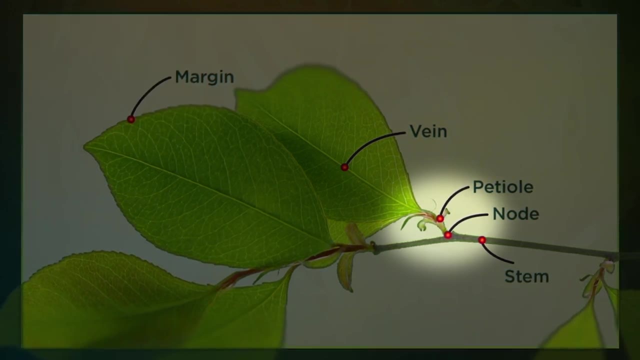 between where the petiole inserts and the main stem. there will be a very small leaf bud there If the structure is a true leaf, if it's a leaflet, there will not be one of these leaf buds Because the bud is located in the axle. 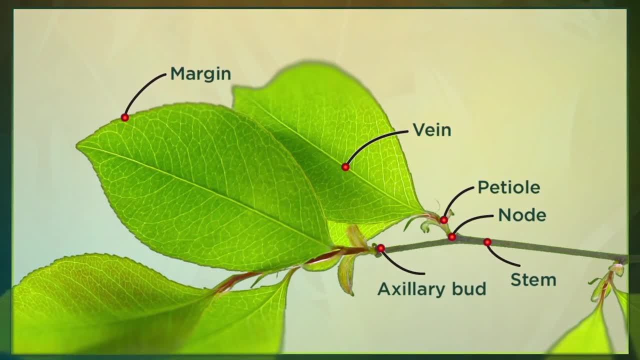 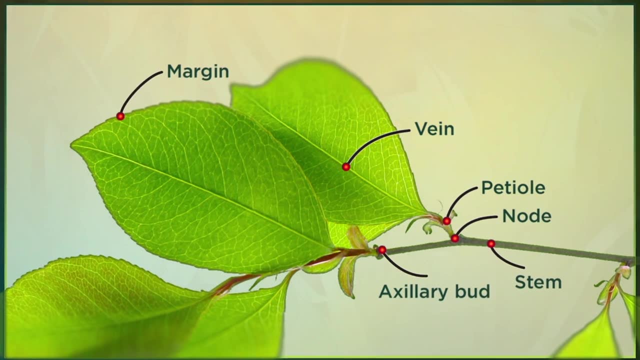 it is called the axillary bud. In anatomy axillary means armpit, So this is sort of like the armpit of the plant, where the stem functions as the body and the leaf petiole is like an arm When the leaflets are arranged like a feather. 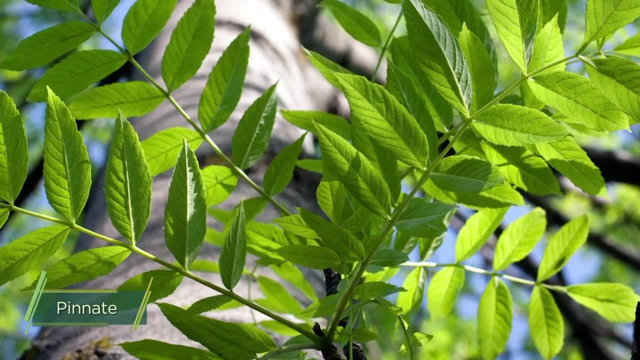 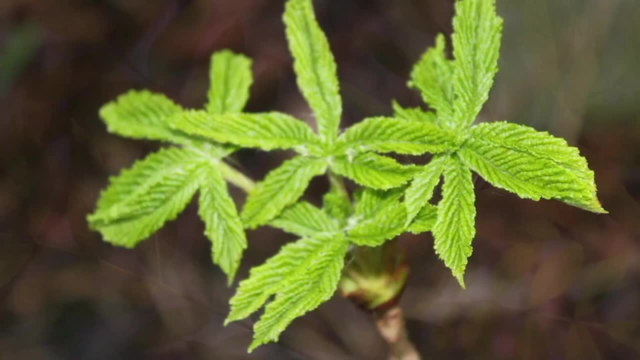 they are called pinnate from the Latin pinnatus, meaning feathered. Common example here would be the leaves of an ash tree. When the leaflets are arranged around a central axis, like your fingers around your palm, the leaf is called palmate. 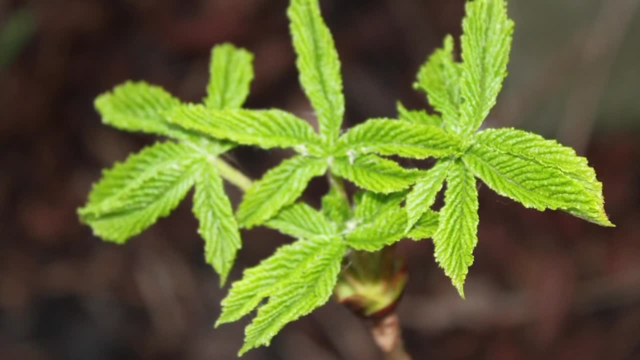 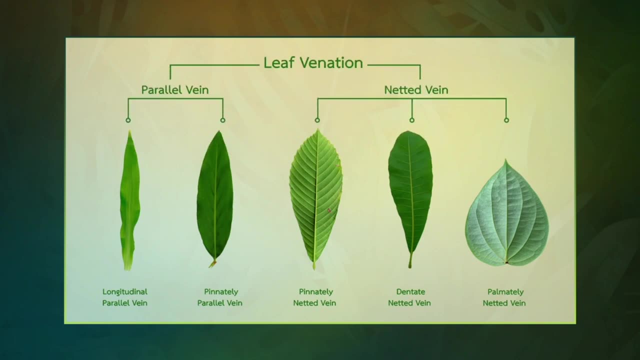 An example of palmate leaves would be the horse chestnut. These terms, pinnate and palmate, are also used to describe the leaf venation, which refers to the arrangement of the veins within the leaves. The veins of the leaves contain the venation. 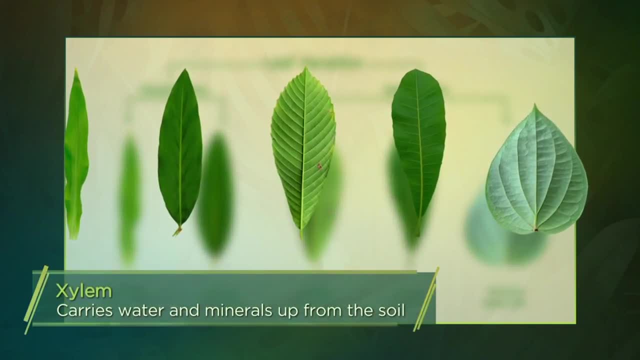 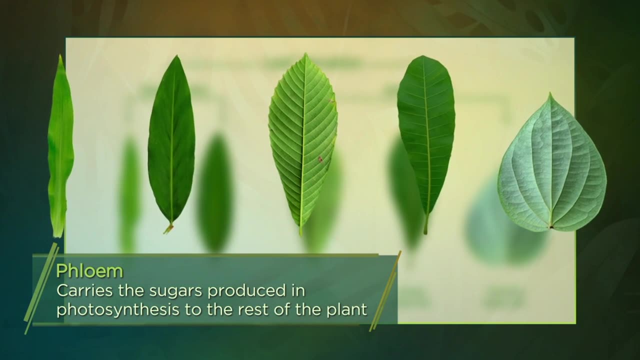 vascular tissue, which is the xylem and phloem. The xylem carries water and minerals up from the soil and the phloem carries the sugars produced in the leaves by photosynthesis to the rest of the plant. Leaf venation can also be linear. 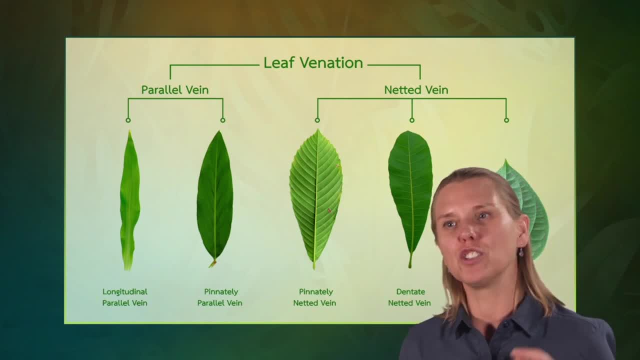 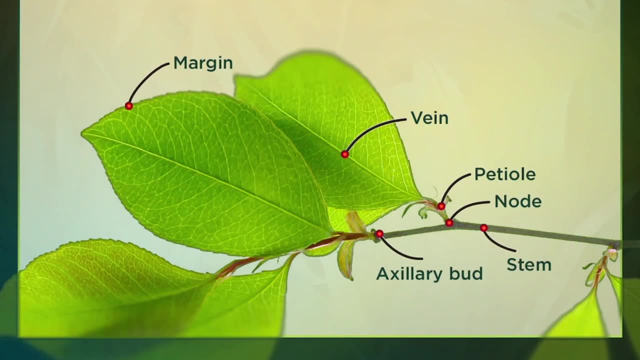 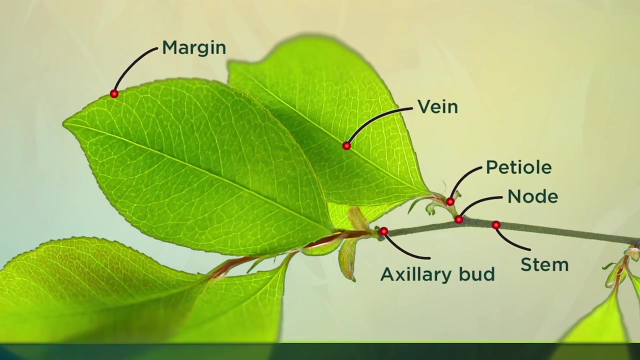 like the veins in blades of grass, And this trait is usually limited to a particular group of plants called the monocots that we'll meet in a future lecture. The last two leaf traits important for identification are leaf margins and leaf hairs. The margin of the leaf refers to the outer rim of the leaf. 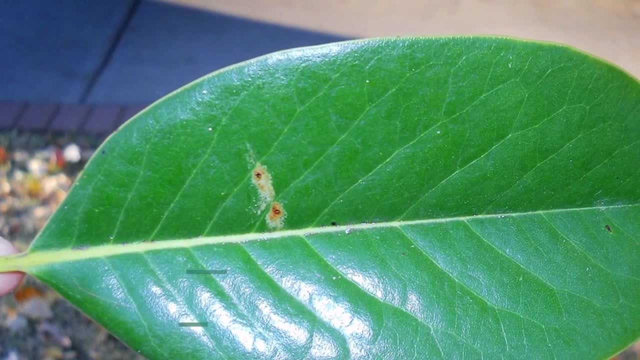 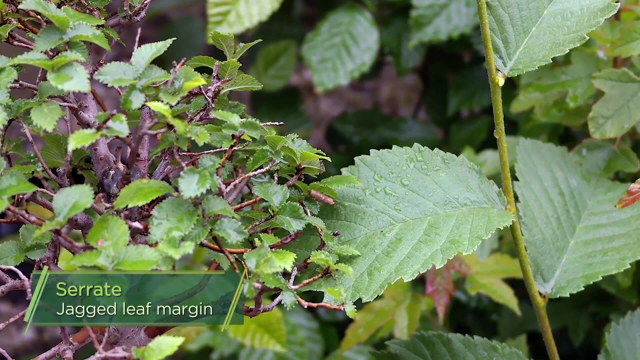 and that can be a defining character. If the leaf margin is smooth, as it is in a magnolia, then it's called entire. If it's jagged in some way, like in an elm, it's given a different name. But the most common of these leaf margin terms 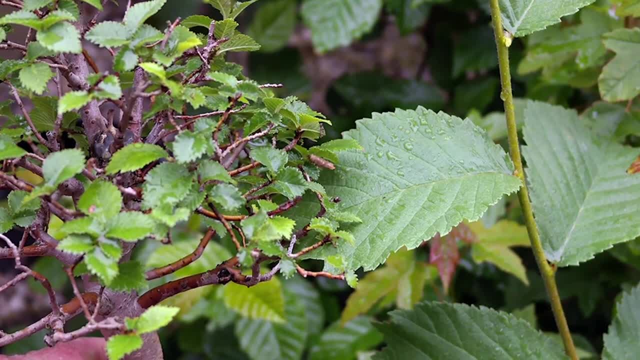 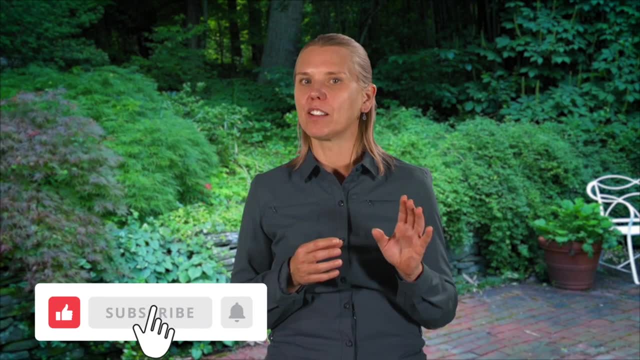 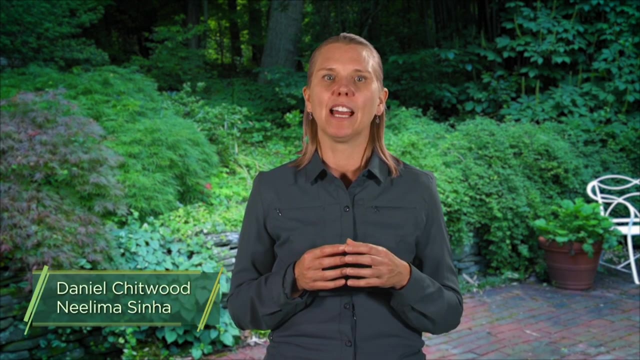 is serrate, which does indeed look like a serrated knife At the edge of the blade. When you look at these leaf serrations, you might wonder why the leaf would do that. In a 2016 review article in Current Biology by Daniel Chitwood and Nalima Sinha, 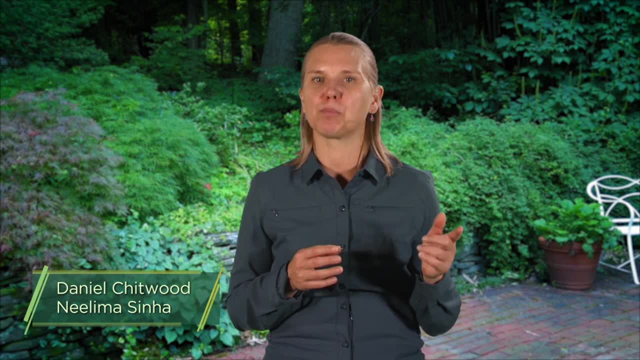 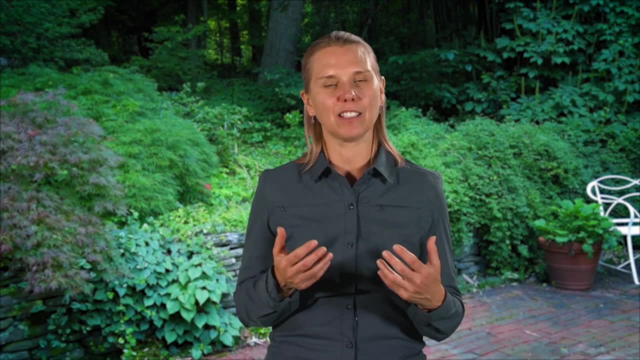 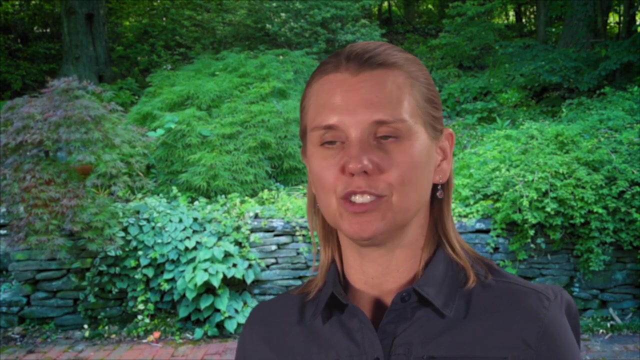 it suggests that there is a trend of more entire leaves being found in the tropics and in the Arctic. The mid-latitudes, it seems, have more leaves with dissected or non-entire margins, While there are several hypotheses for why this trend might exist. there's no definitive answer yet. It could be that leaf dissection is a good way to let light down to the lower levels in a tree's canopy. or it could be that leaf dissection is an easier way to get your photosynthetic machinery up and running. 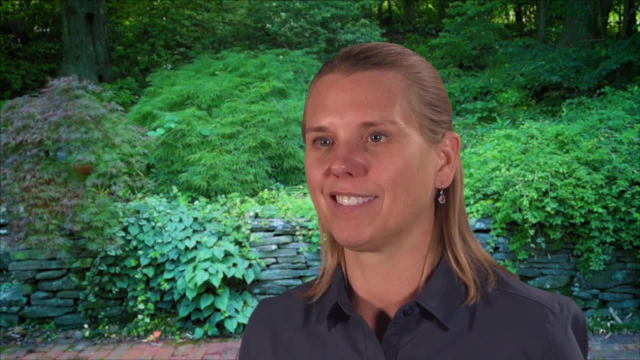 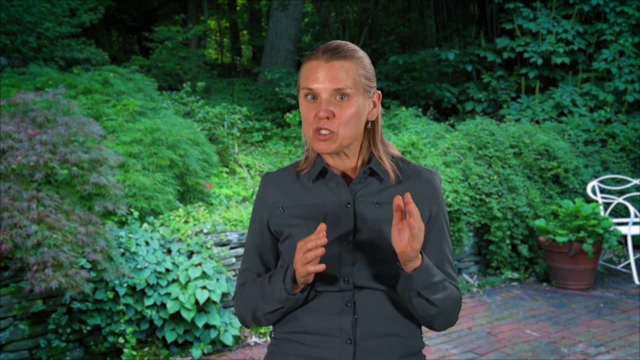 during the growing season. without producing an entire leaf, Ha Get it Entire leaf. As for our last distinguishing trait for leaves, usually just the leaves, Usually just the presence of leaf hairs is enough. Botanically, leaf hairs are referred to as trichomes. 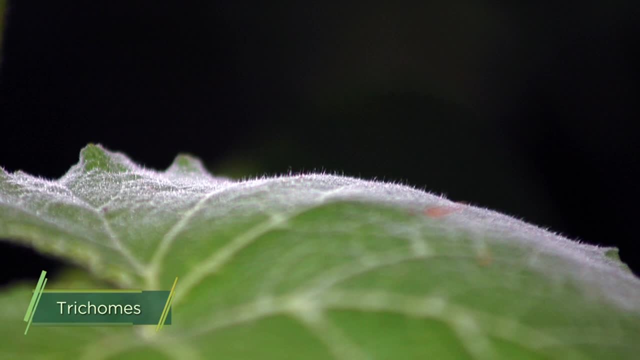 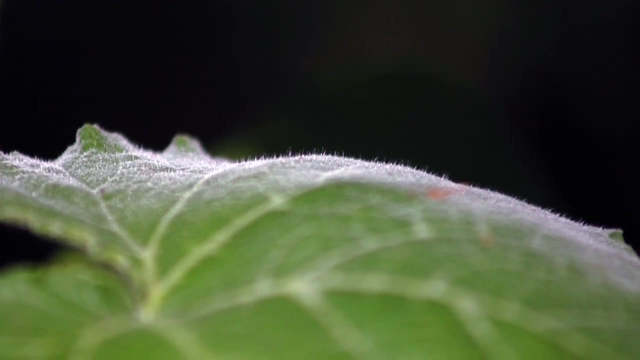 and, unlike leaf, margin shapes. the function of trichomes is well known. The hairs on leaves work a lot like hair on animals. The trichomes can regulate leaf temperature and also serve as a glandular outlet for chemicals that will protect the leaf from herbivory. 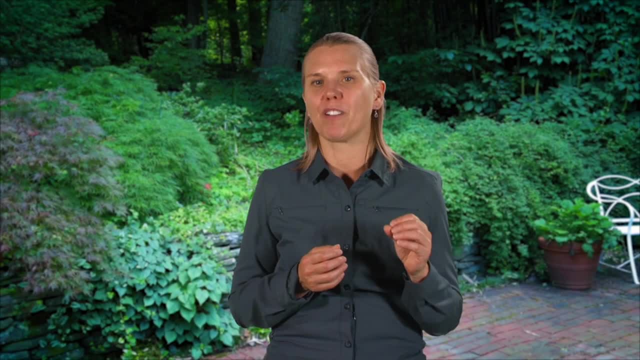 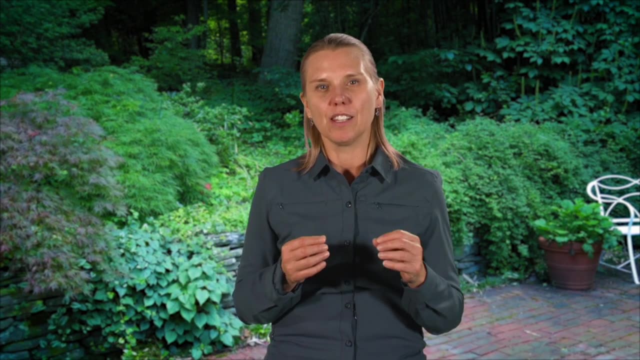 usually from insects. The trichomes can also help prevent water loss by increasing the amount of water in the leaves, By increasing the boundary layer of air around the leaf. Essentially, this means that the wind speed near the leaf will be slower and this will slow evaporation of water. 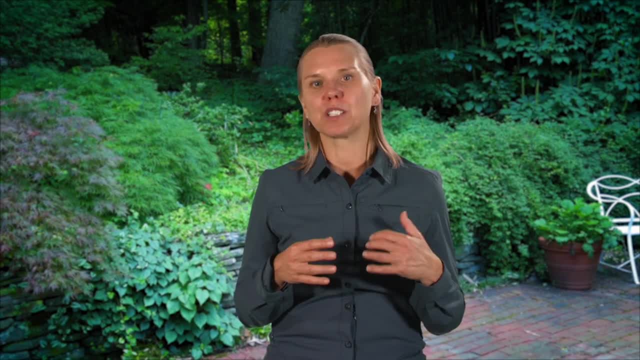 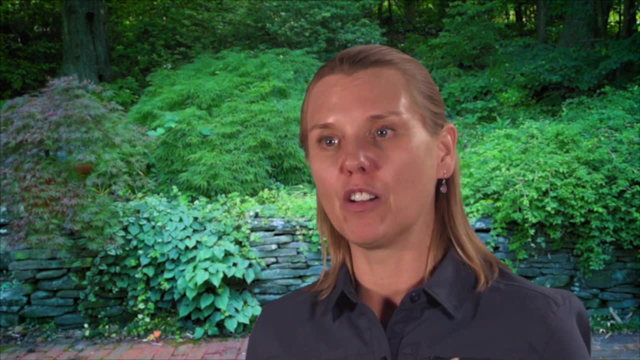 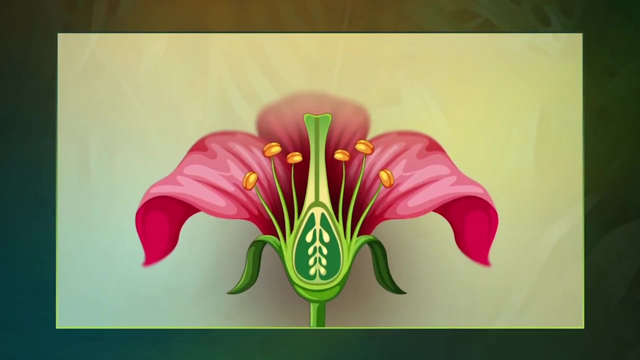 out of the leaf. Lastly, trichomes can serve to protect the leaf against too much solar radiation, Moving up the plant on our terms to know for plant identification. we come to flowers. Though we covered flowers in chapter three, they are so important to us. 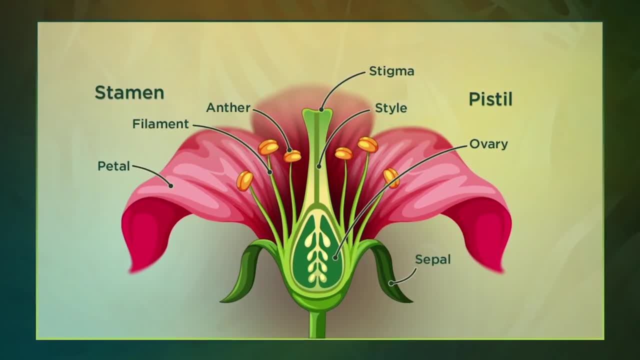 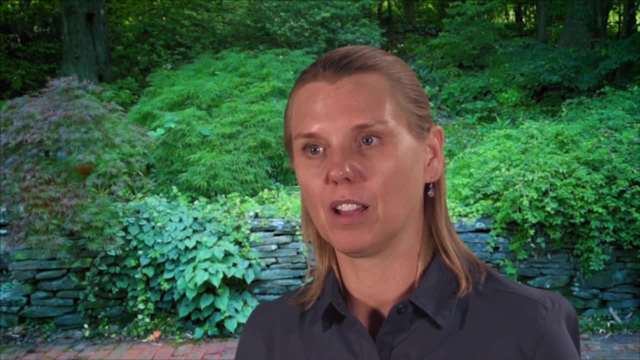 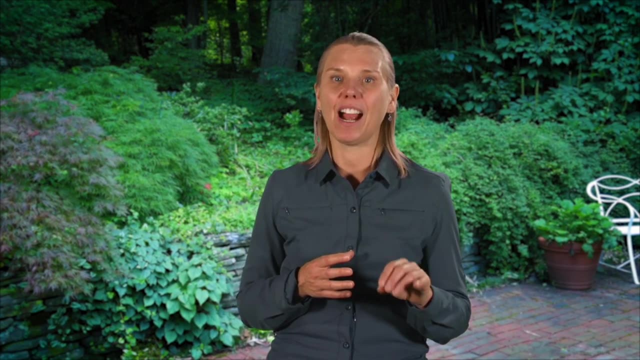 They will also be the basis for all fruits that the plant will form. However, wherever there is a flower, there isn't a guarantee of a fruit. That flower has to be pollinated, That is pollen, which carries the sperm of the plant. 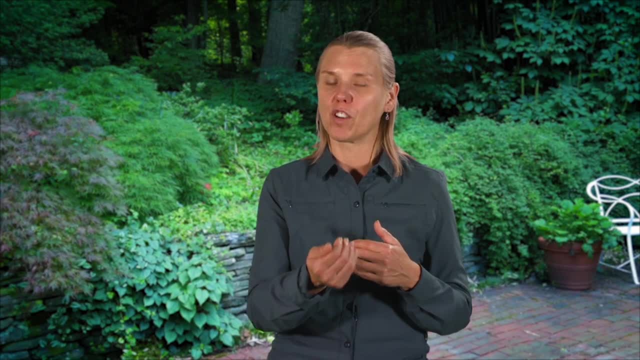 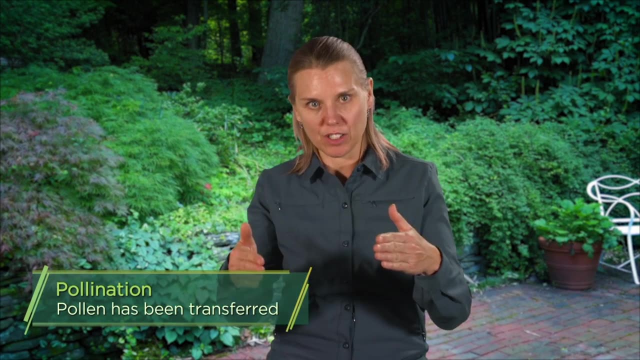 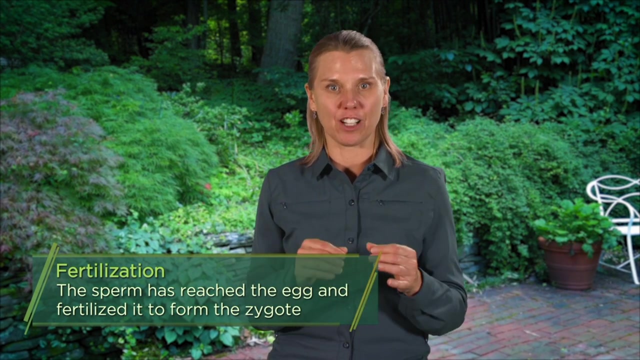 must reach the pistil of the plant in order for fertilization to occur. These two words are not synonymous: Pollination means pollen has been transferred, and fertilization means that the sperm has reached the egg and fertilized it to form the zygote. 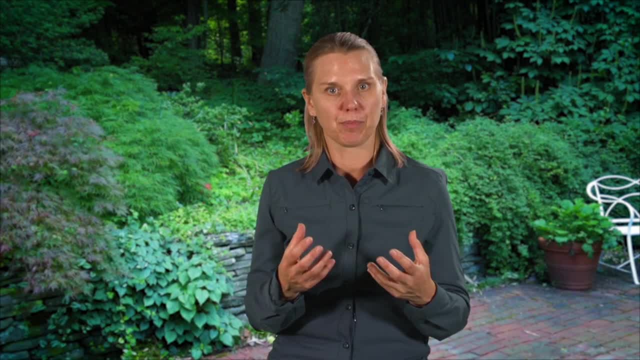 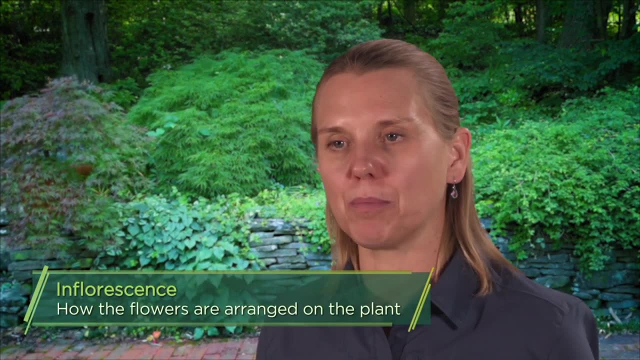 which develops into the embryo inside the seed. Before we even investigate the structure of the flower, we can observe how the flowers are arranged on the plant. This arrangement is called the inflorescence, and the type of inflorescence can be very different. 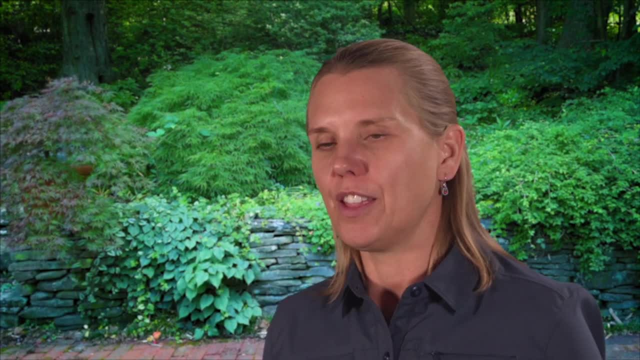 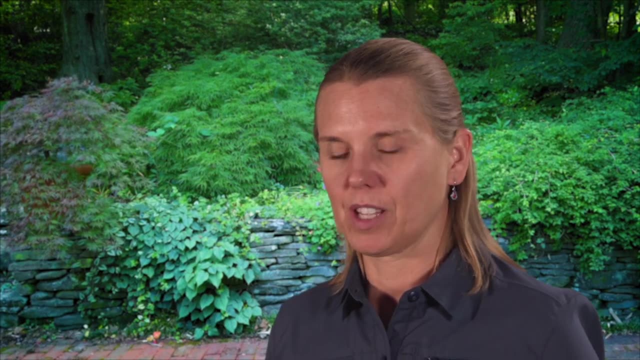 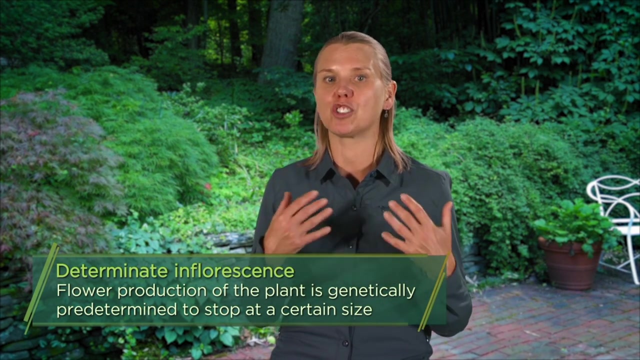 and very important in determining plant families. There are two main categories of inflorescences. They can be determinate or indeterminate. A determinate inflorescence is one where the flower production of that plant is genetically predetermined to stop at a certain size. 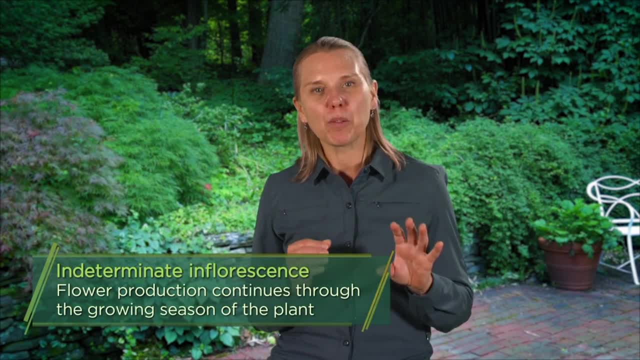 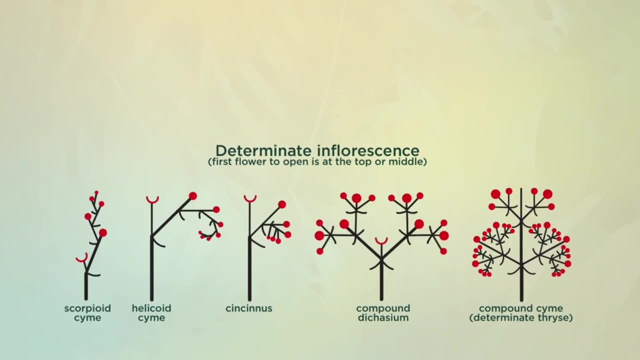 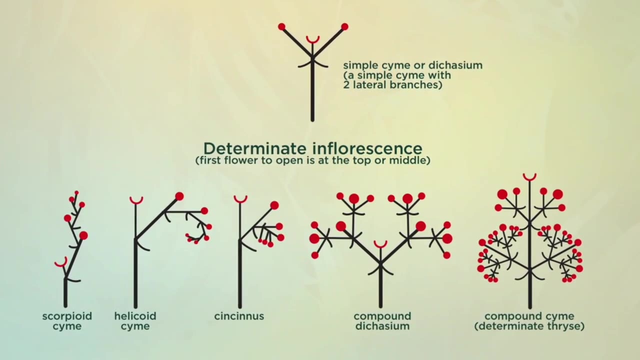 An indeterminate inflorescence is one where flower production continues through the growing season of the plant. The main determinate inflorescence types are all a variation on a cyme, which is an inflorescence where the central flower develops first. 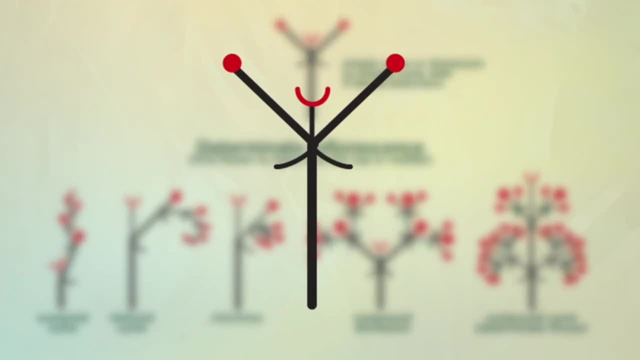 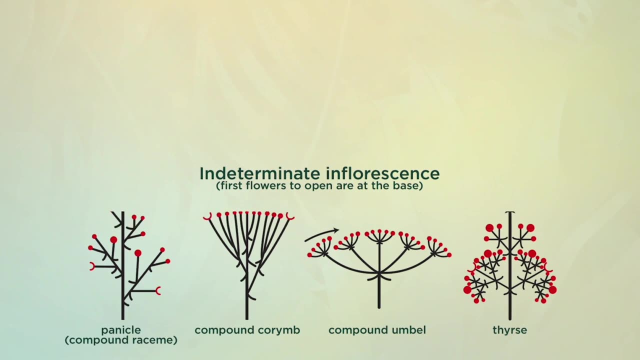 In the figure, the half-moon shapes are the flowers that are first to open. Indeterminate inflorescences are a bit more varied. The first flowers to open are at the base and as the plant continues to grow up or out. 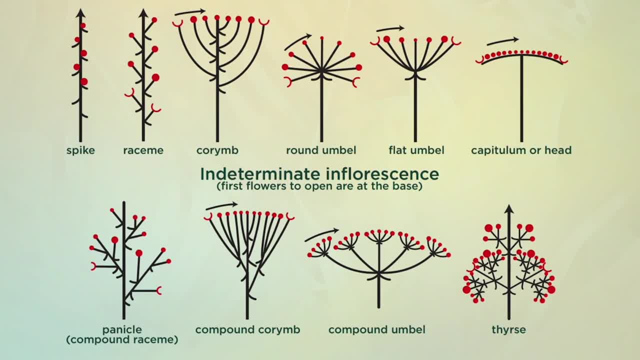 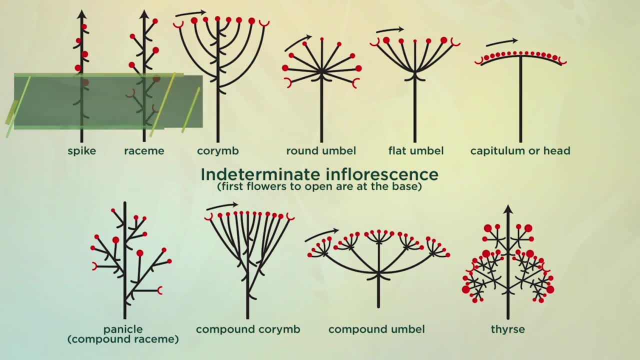 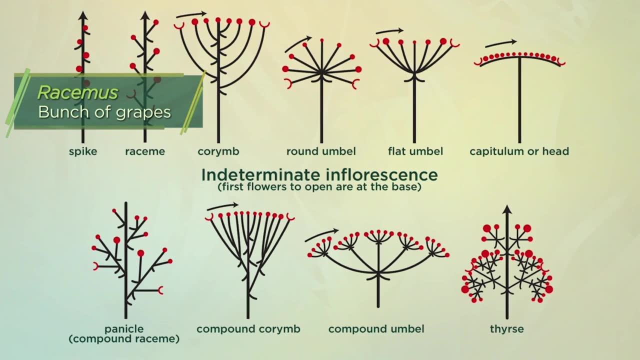 more flowers develop. The most common indeterminate inflorescence is a raceme, like foxglove or lupine. This word comes from the Latin word racemus, which means bunch of grapes. I'm not sure a raceme looks like a bunch of grapes. 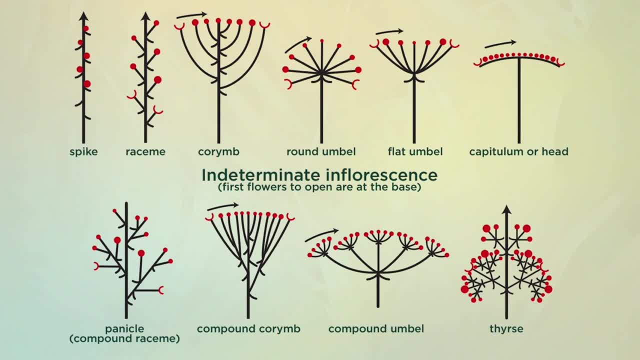 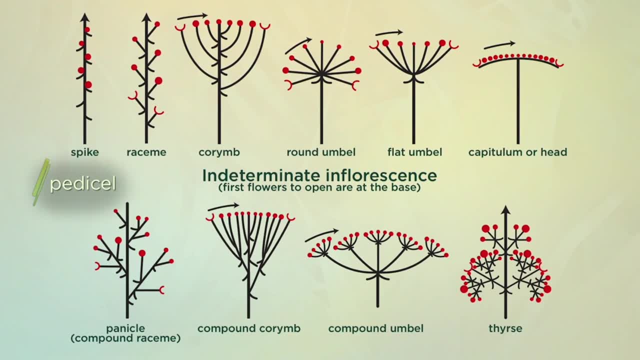 but there are many flowers and they alternate up the stem. The flowers will be on a small stalk called a pedicel, And if there is no pedicel but the flowers are on either side of the stem, then the inflorescence is called a spike. 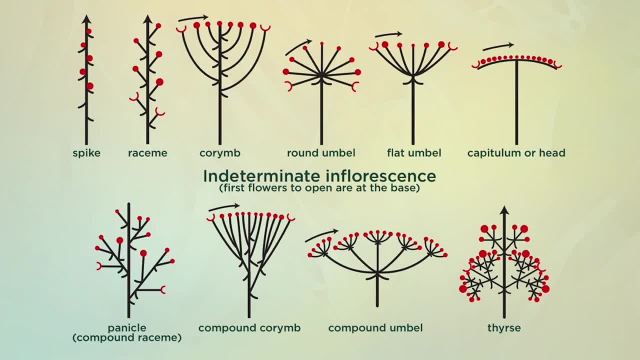 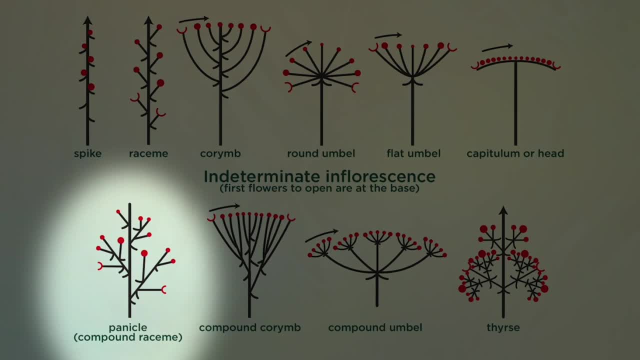 If there is more than one flower coming off of the stalks, then the inflorescence is a compound raceme or a panicle, And a good example here is a lilac, If the flower stalks all join to a central location. 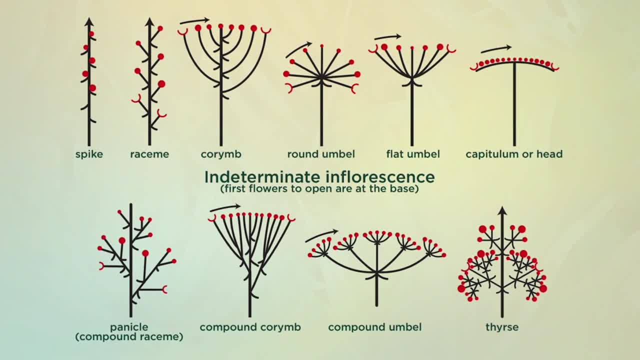 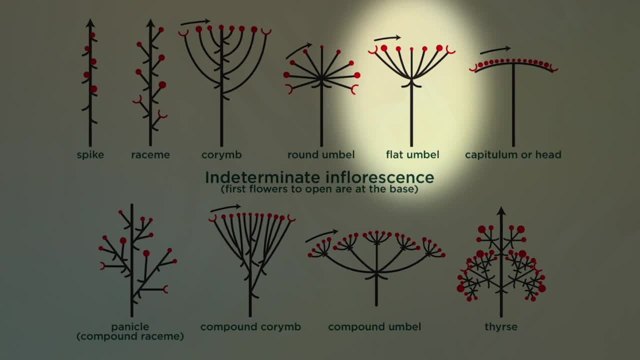 on the stem to form an upside down umbrella shape. this inflorescence type is called an umbel, from the Latin umbella, meaning sunshade or parasol, And, lucky for us, this is the same root as umbrella, So the umbel inflorescence. 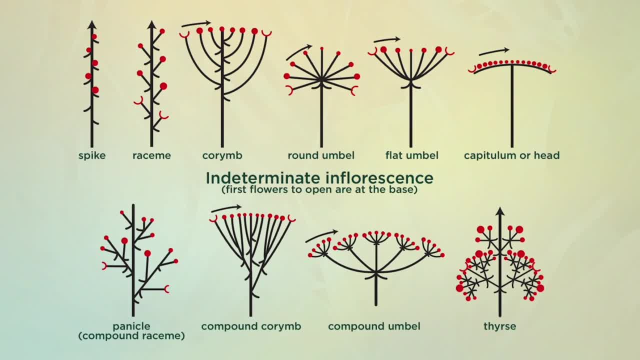 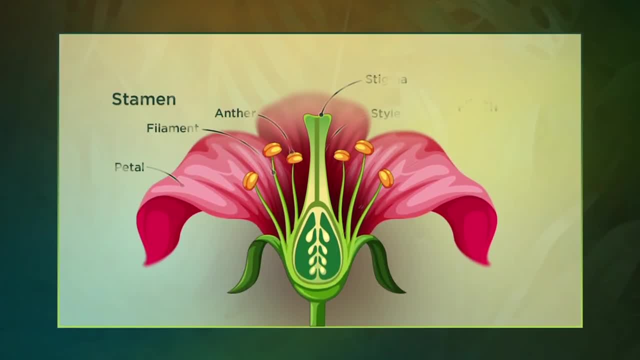 should be easy to remember. Umbel is an upside down umbrella. A good example of an umbel is wild carrot. If we continue our discussion of distinguishing terms, we can explore the flower itself, Moving from the bottom to the top of the flower. 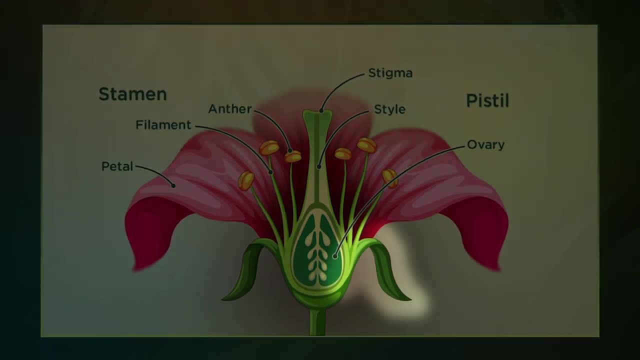 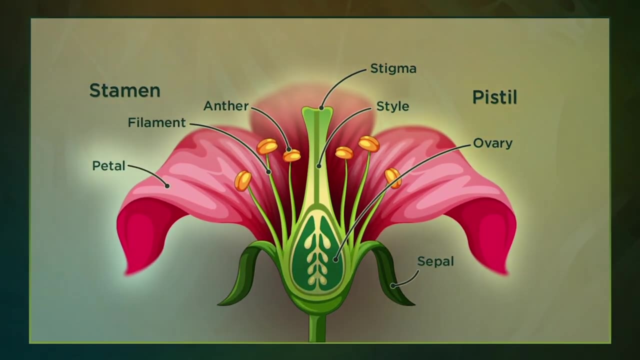 we begin with the green leaf-like structures that are just below the colorful petals. These sepals usually form the outermost part of the flower bud. The petals are typically the ones that form the flower bud. The petals are typically the ones that form the flower bud. 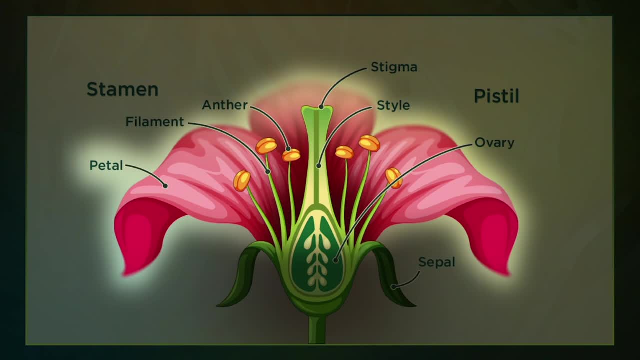 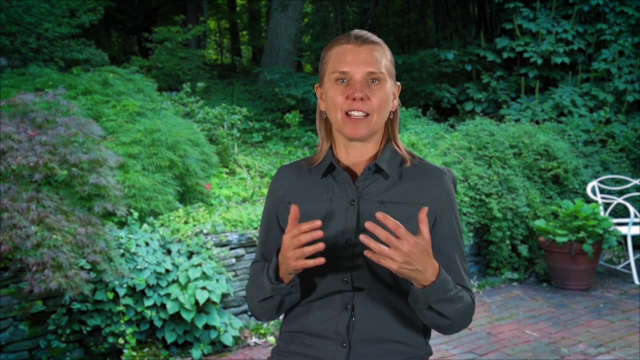 The petals are typically colored in order to attract pollinators, which are animals that will transfer pollen from one plant to another. If the flowers are showy, which means typically that they're noticeable and colored, then they are usually animal pollinated. 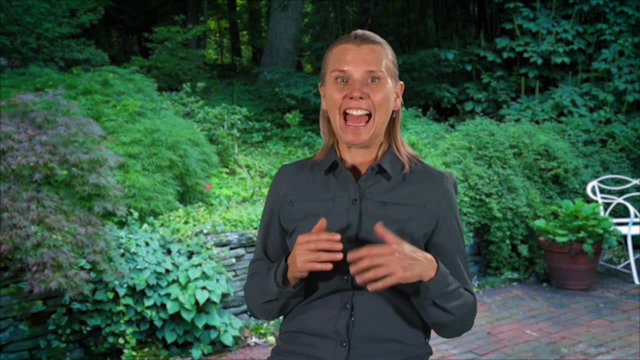 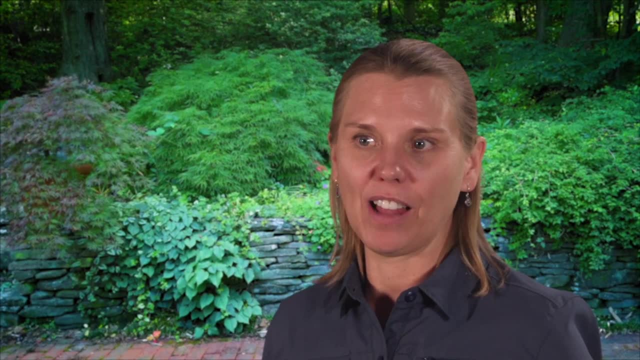 Some flowers, by contrast, are decidedly not showy and lack much color, and these flowers tend to be wind pollinated. An example of an animal pollinated flower is this pretty scarlet helia or Ipomoea or Ipomopsis aggregata. 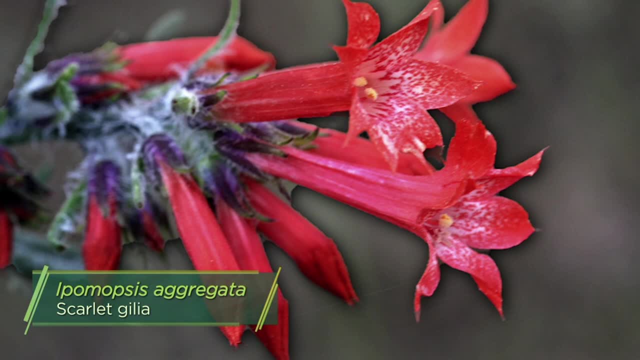 Its red color signifies that it is attracting a pollinator, and the long tube shape of the flower tells us that it's pollinated by an animal with a long tongue, such as a butterfly or a hummingbird. An example of a wind pollinated flower: 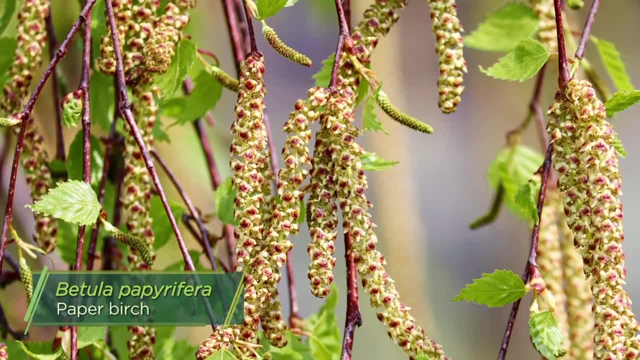 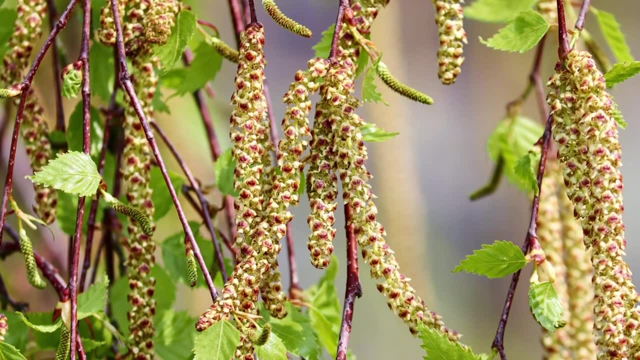 is this paper birch, Betula pepifera. This flower is inconspicuous and small. The flowers have no bright color or smell, and that's because these flowers don't need to attract insect pollinators. There are numerous descriptive terms. 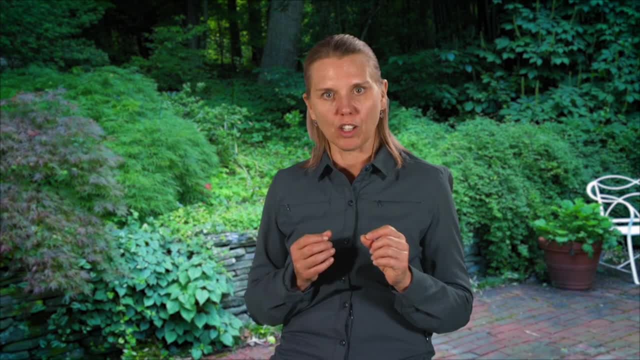 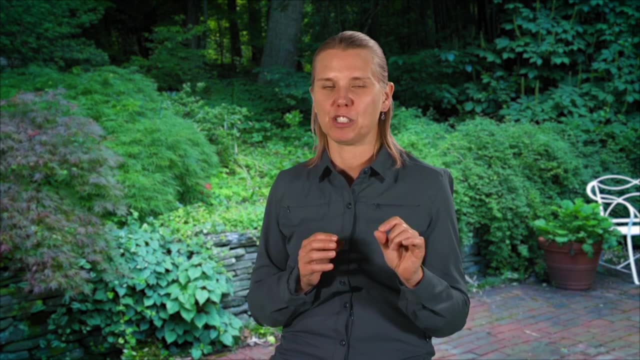 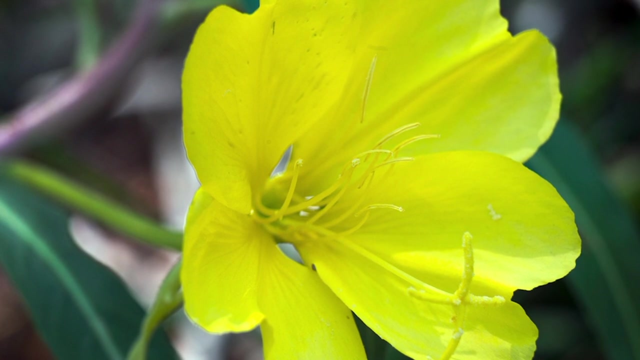 for the overall shape of the flowers. We'll start with overall flower symmetry. This is an important diagnostic character and there are three different symmetry types for flowers. If the flowers can be dissected in multiple planes like a pizza, it has radial symmetry. 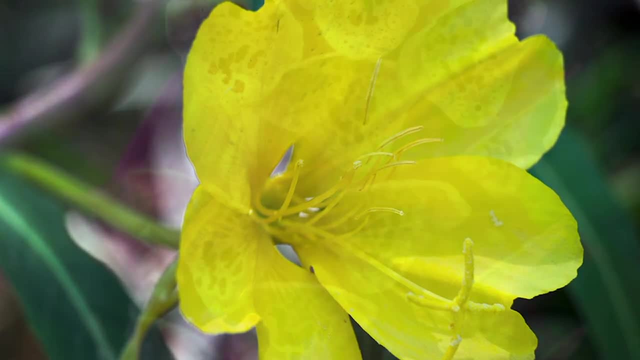 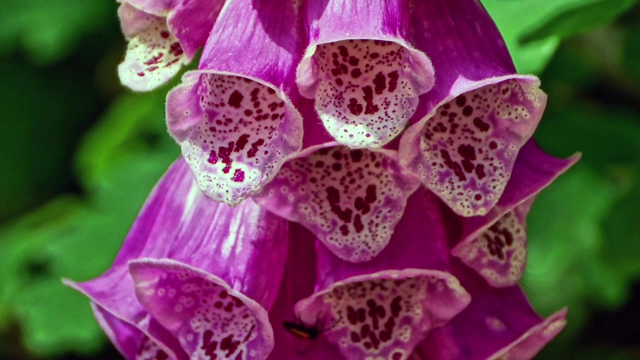 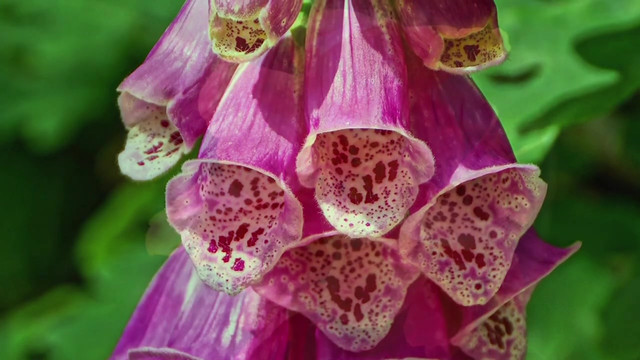 An example is this evening primrose. If, like a human, there's only one way the flower can be dissected to reveal two symmetric halves, then it has bilateral symmetry. An example is this digitalis flower. Lastly, some flowers have no symmetry. 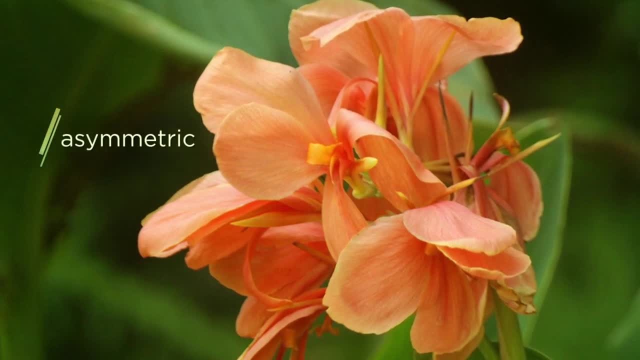 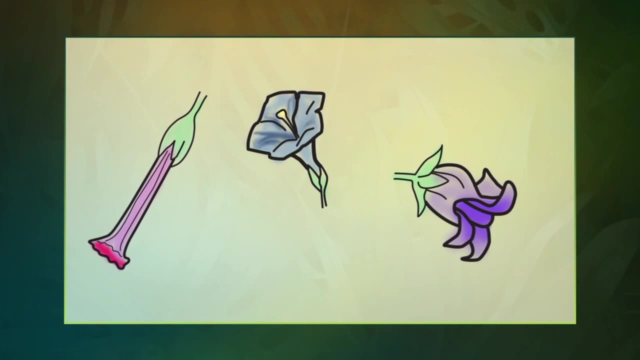 like members of the canna genus, and these are called asymmetric Like leaf shape. there are many different names for the shape of the petals. Collectively, the petals are referred to as the corolla and they are the most common names for the petals. 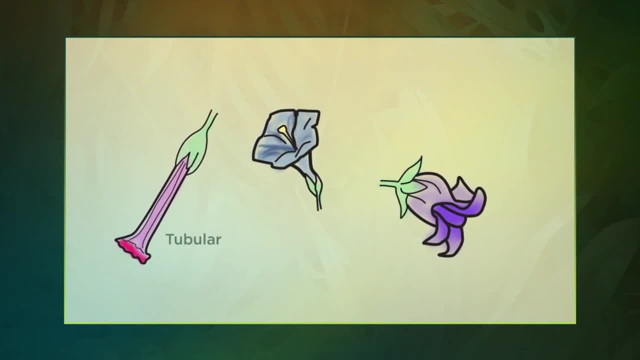 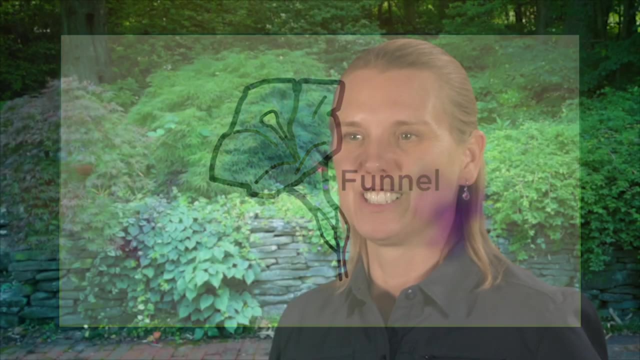 and some words used to describe the corolla are tubular, trumpet-shaped and funnel-shaped. Each of these is a variation on the theme. tubular, The trumpet shape flares out at the end and the funnel-shaped flares out even more at the end. Rather than define every floral type here, 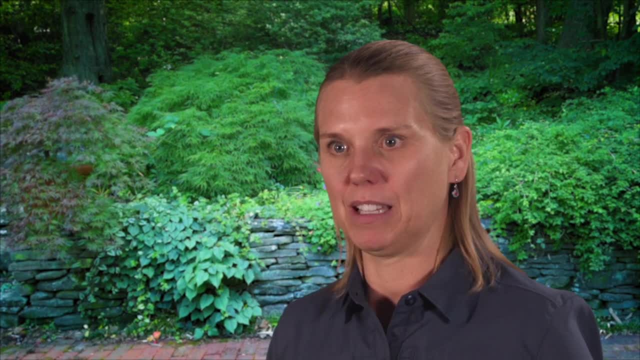 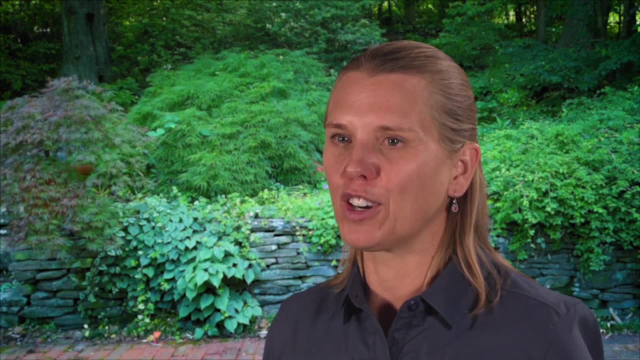 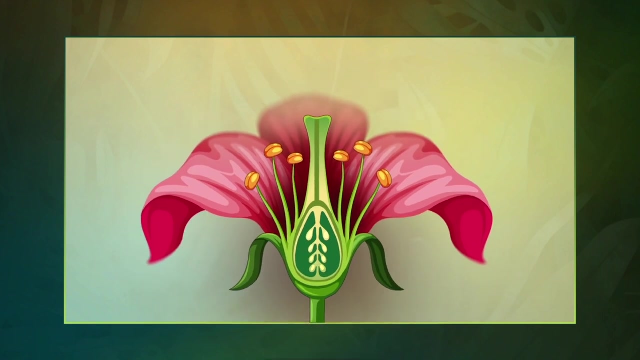 I'll introduce important floral shapes as we meet them, and most identification books will have a glossary. While most of these botanical terms are universal, it never hurts to see just what the exact definition is for the identification book you're using. Moving to the inside of the 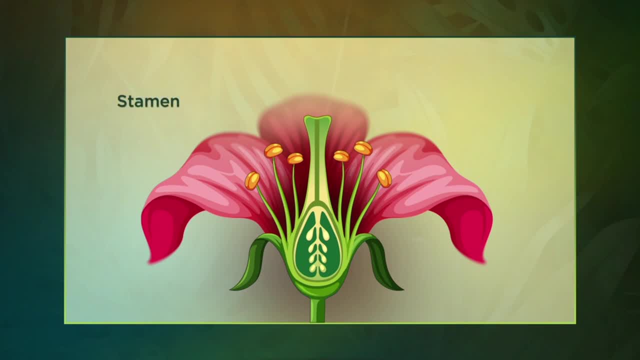 petals. we come to the male parts of the flower, or the stamen. They are comprised of the anther, which sits on the filament. Usually it's the number of stamen that we're concerned with in identification, so we'll leave it at that for now. The pistil is the female portion of the flower. It 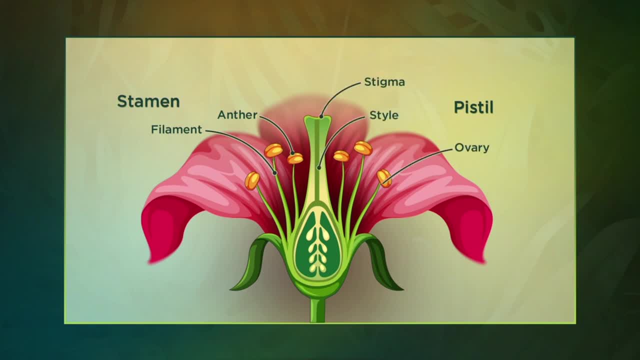 contains the stamen. The pistil is the female portion of the flower. It contains the stamen, Sticky stigma at the top, where the pollen lands, and a long style that goes down to the ovary, Where the ovary sits. in relation to the rest of the petals and sepals collectively. 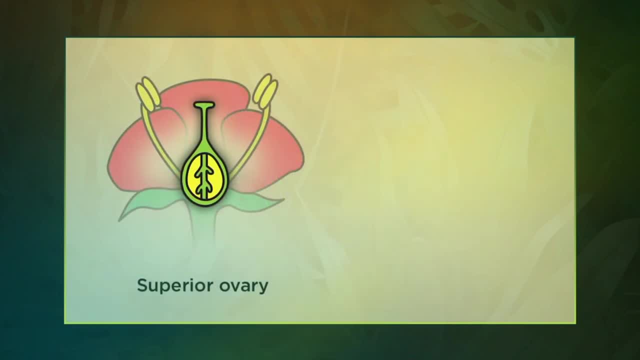 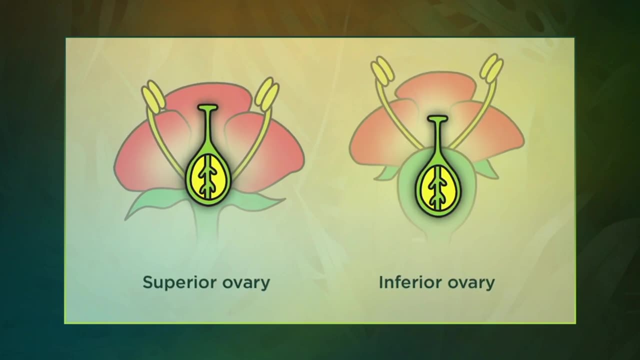 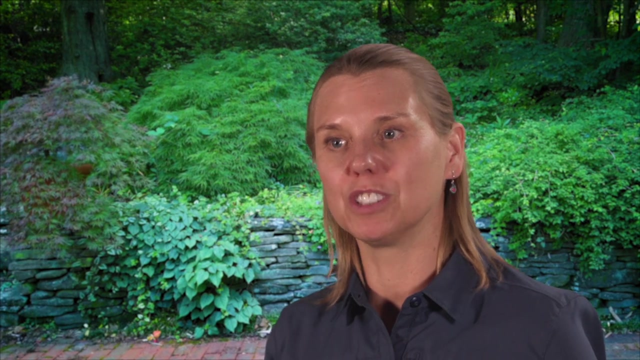 called the perianth, will be important. A superior ovary sits on top of the petals and sepals and an inferior ovary sits below the petals and sepals. Some plants have more than one pistil. Determining the number of pistils is important to 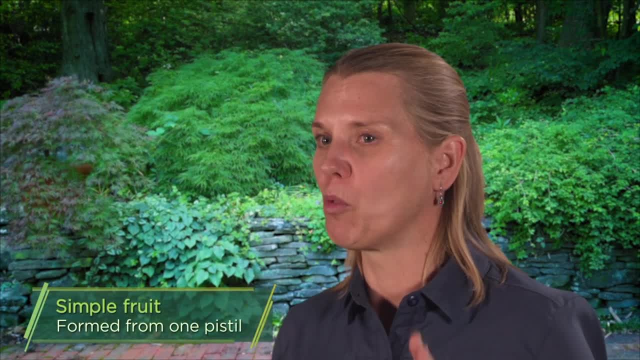 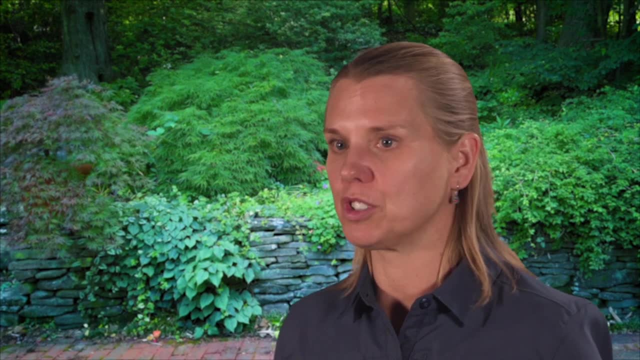 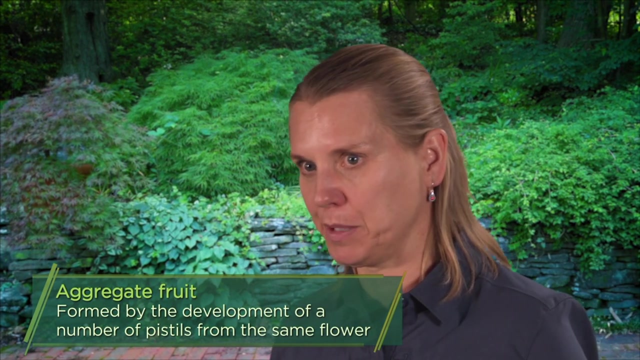 distinguishing the fruit type. Fruits that are formed from one pistil are called simple fruits. This is the most common fruit type, and just a few examples are apples, oranges, tomatoes, cherries. An aggregate fruit is one that is formed by the development of a number of pistils from 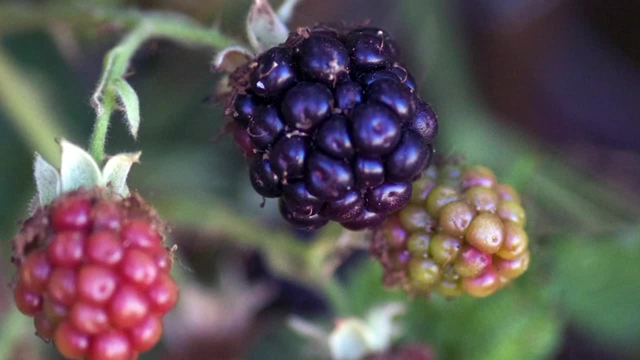 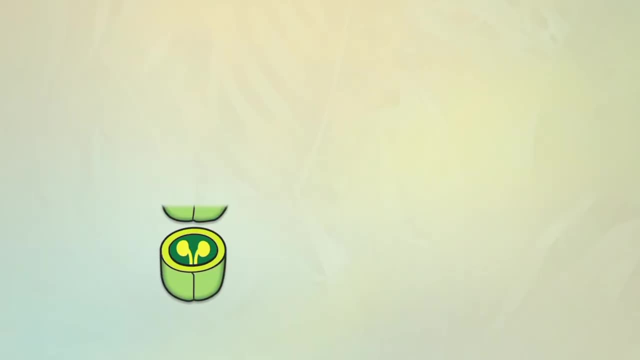 the same flower. An example of this type of fruit is a blackberry, which is an aggregate of many different fruits. The ovary within the pistil can be divided into different segments. The flower is called a monocarpic. The pistil is always formed by only one of its distinct segments. 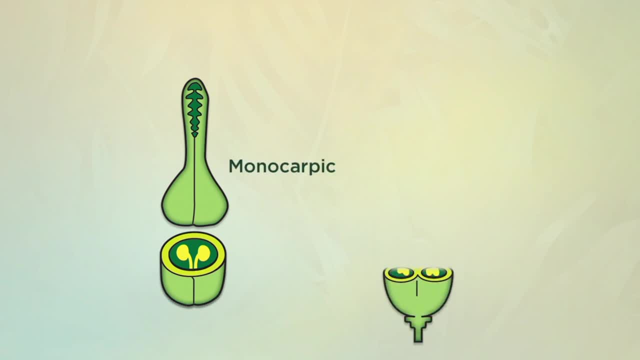 called carpels. If there is just one carpel in the ovary, then the flower is monocarpic. If these carpels aren't fused, then the pistil is the same as the carpel. But if there is more than one carpel and it's fused into one pistil, then the flower is syncarpus Many times the number of 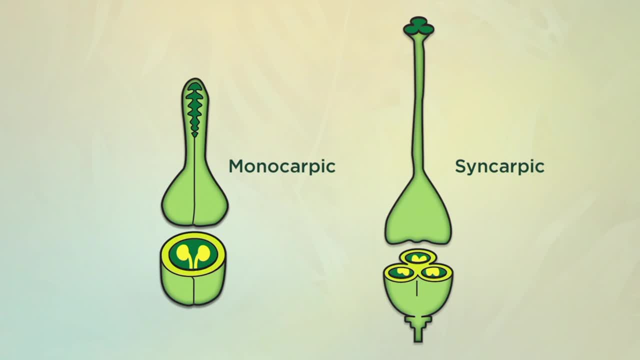 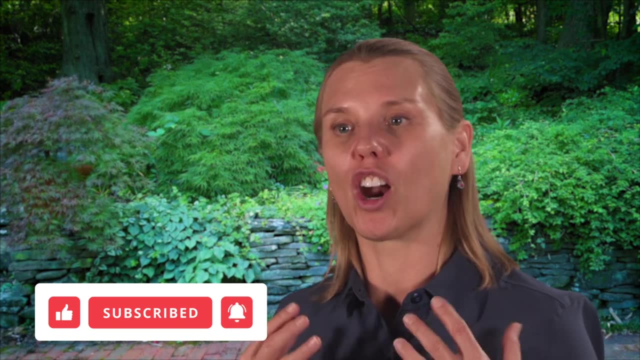 styles or the number of stigma lobes will be a clue as to how many carpels are contained in the ovary. that the ovules, the unfertilized eggs, inside the carpels are attached to the carpal wall is also important for some families. Now we've used the words carpal. 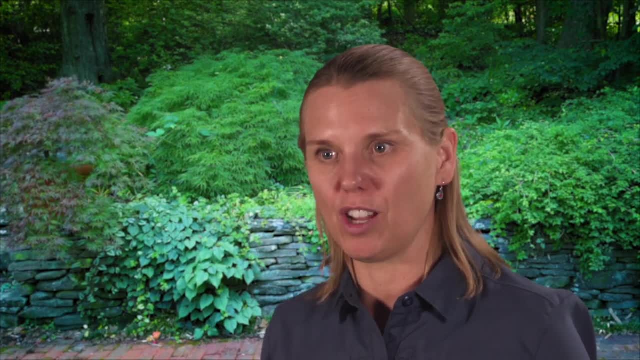 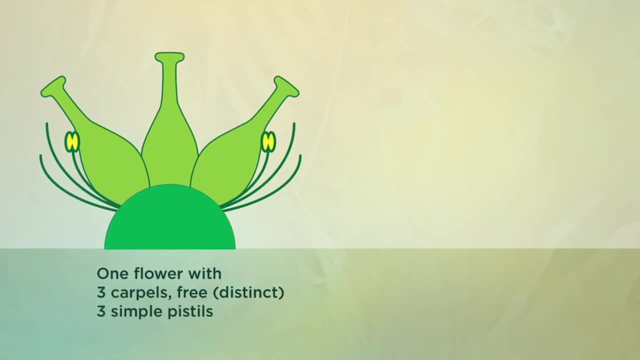 and pistil, and sometimes these mean the same thing, but other times they don't. For example, you can have one flower with three unfused carpels and three simple pistils, but it's also possible for a flower to have three fused carpels and. 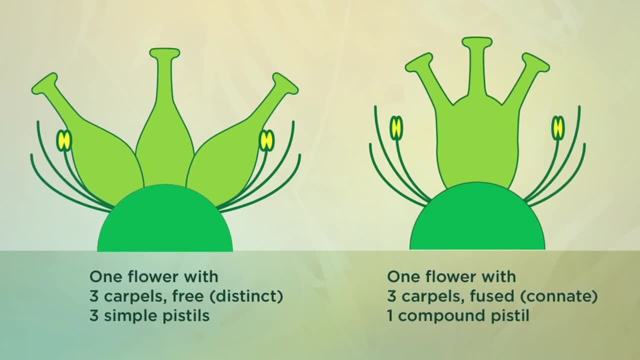 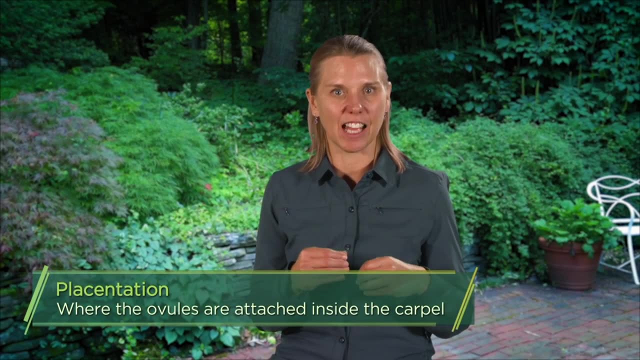 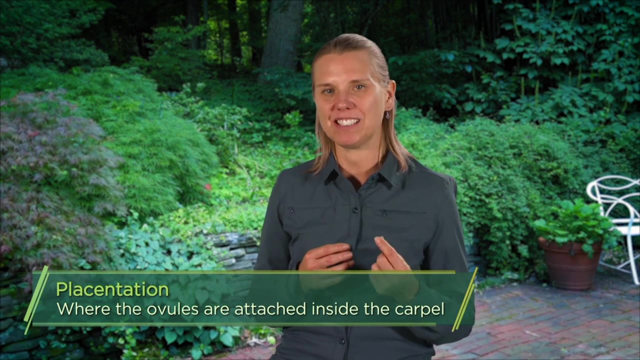 also three styles and three stigmas. but since the carpels are fused, there is only one pistil Where the ovules are attached. inside the carpel is called placentation. Again, placentation becomes more important when determining species. 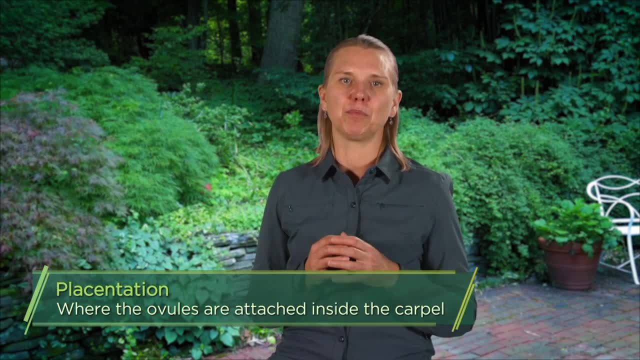 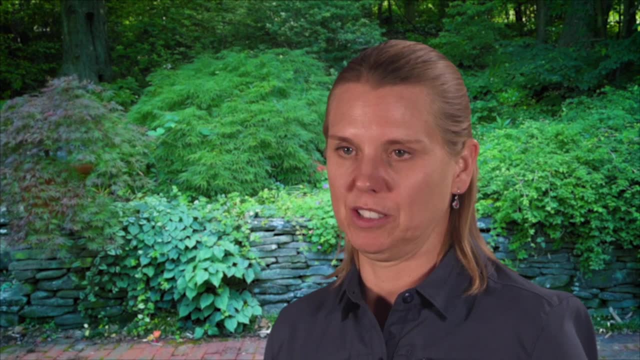 or genera rather than families, so you needn't commit them to memory, Just be aware of their existence. As we discussed, the ovary is where the inviol is contained. The ovule is the place where the ovule is contained, So the ovule is. 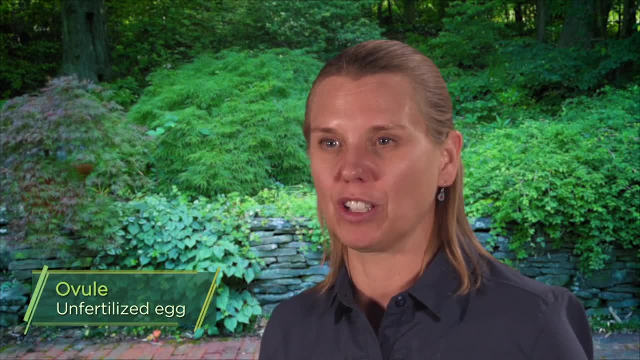 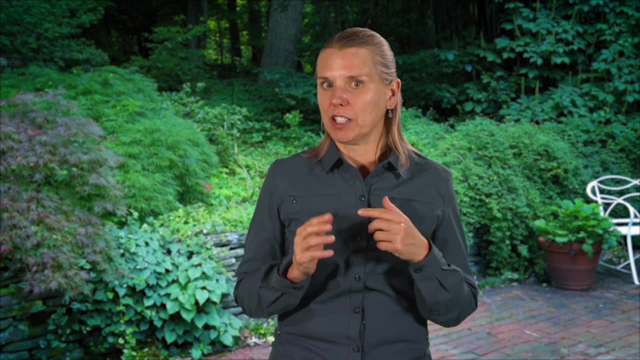 the place where the ovules exist. The ovule is where the allied ovules, if they're the name for the unfertilized egg. When that egg is fertilized, the embryo begins to form inside the developing seed. There may be more than one ovule in a carpal and more than one 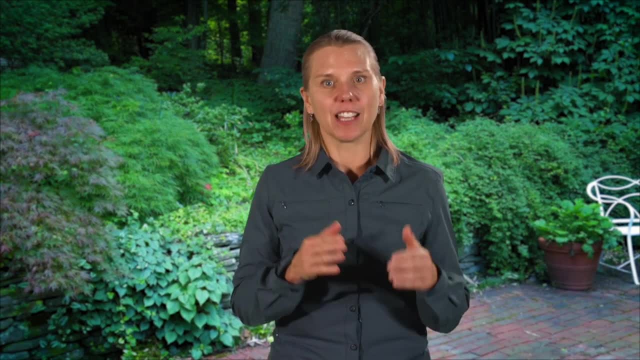 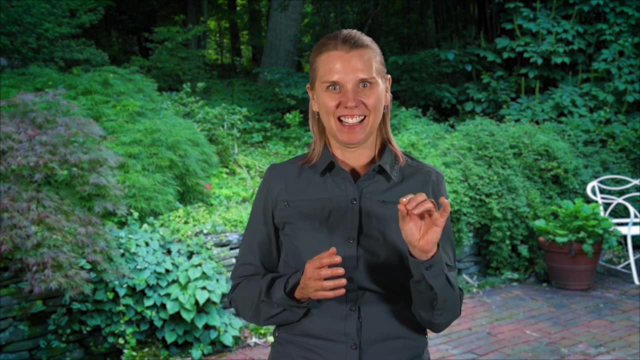 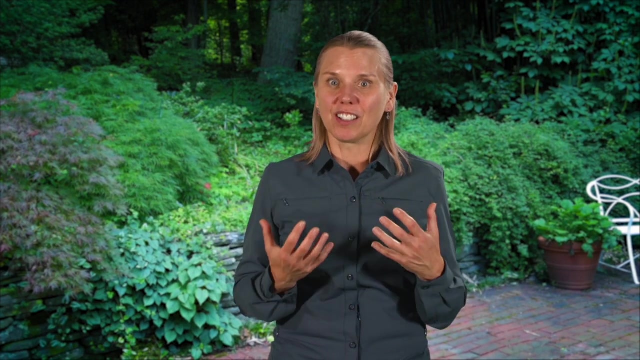 carpal in an ovary. Most fruits are simple fruits, that is, they are derived from one pistil. Keep in mind that the fruit is the swollen ovary, And keying out fruit types is actually pretty fun. There are many fruit keys available online and you can collect fruits from the grocery, but 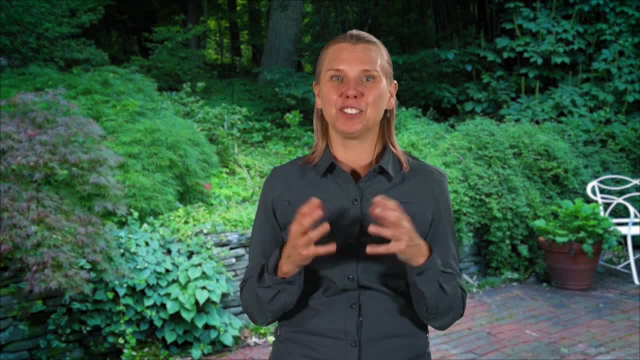 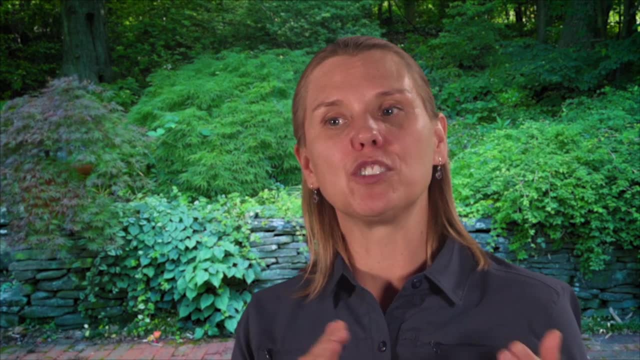 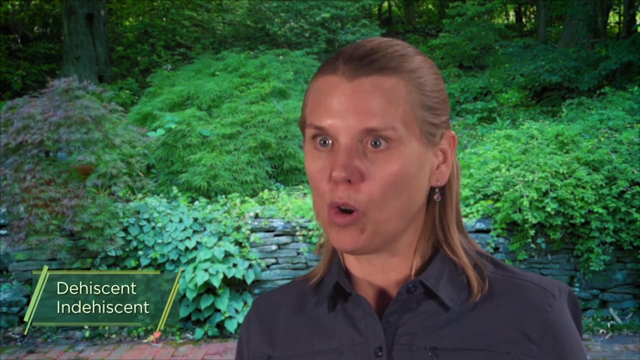 also from the backyard. It's really fun and you get to eat your study specimen when you're done. So simple fruits derived from one pistil can be dry at maturity or fleshy. If a fruit is dry at maturity, it will be dehiscent or indehiscent. That word, dehiscence, is derived from the Latin. 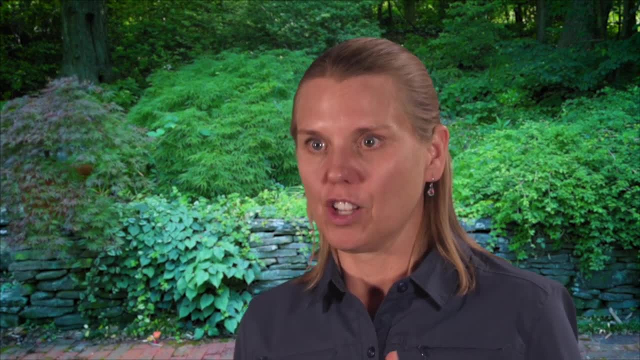 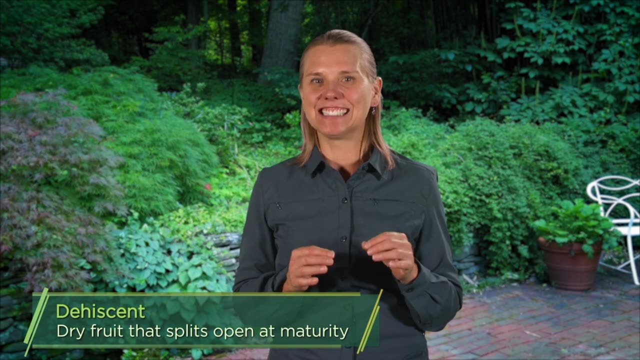 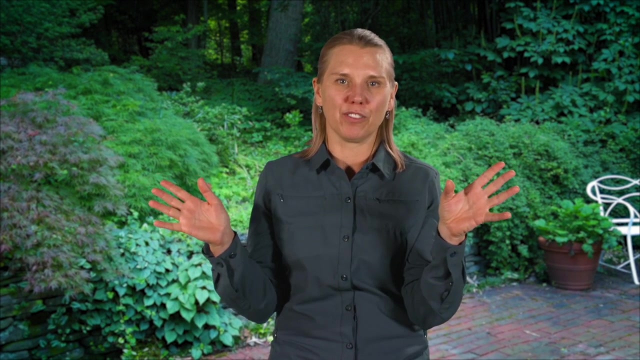 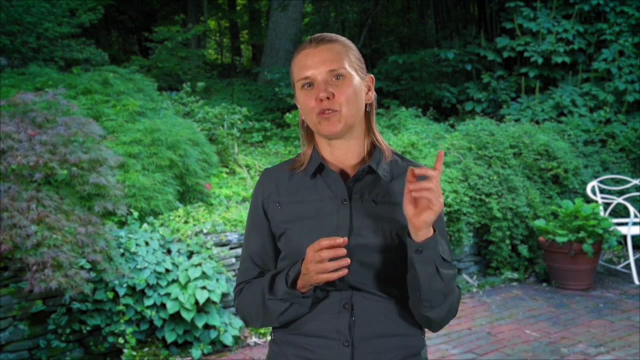 De-his, which means to split, So a dehiscent fruit is a dry fruit that splits open at maturity. I like to think of it as dehiscent, and the hiss sound might remind you of the seed splitting out of the fruit. It may be useful here to think of the 2018 research findings of Dwight Whitaker. 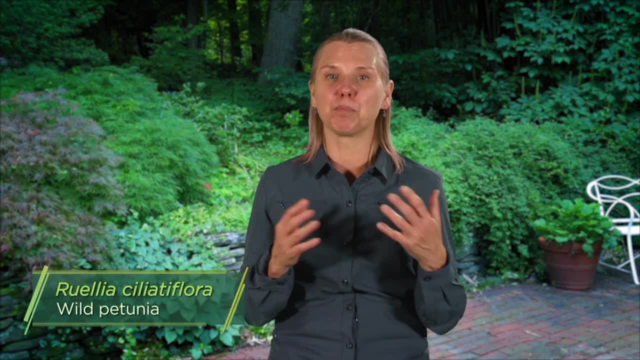 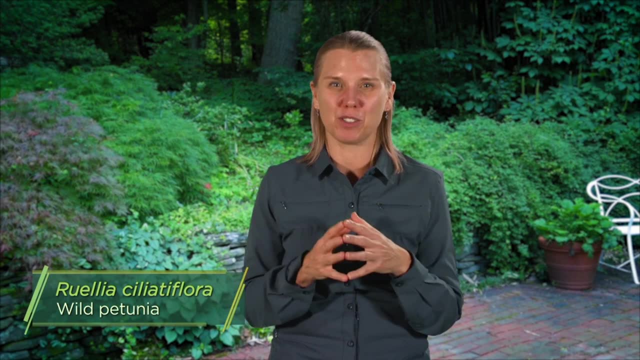 at Pomona College, who found that the seeds of the wild petunia, Rulia, ciliatilla, flora, de-hiss out of the fruit at 15 meters per second, and that these seeds can spin up to 100,000 rotations per minute. 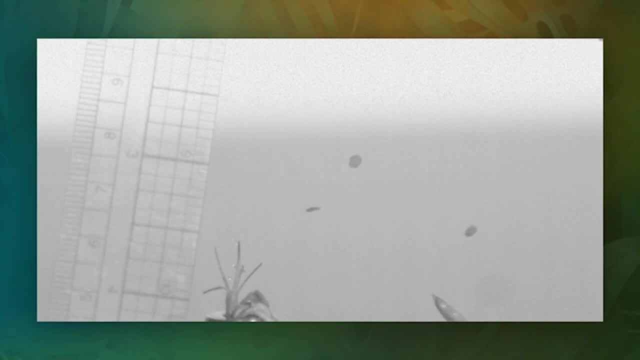 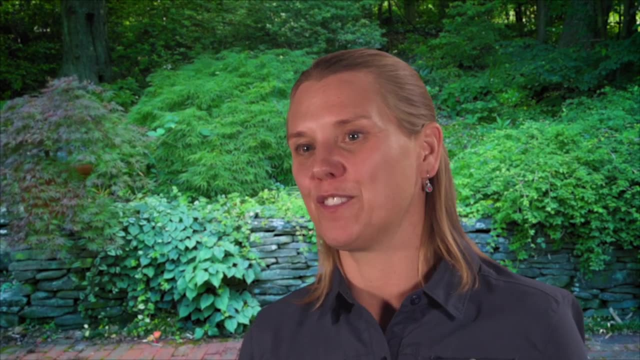 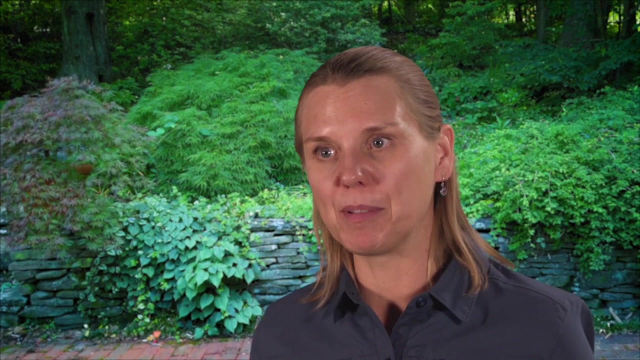 which is the fastest seed travel known. According to the journal Nature, that's the fastest natural projectile known. Let's begin with the dehiscent fruit types. Remember they hiss or break open at maturity to release the seeds. One of the most common is the: 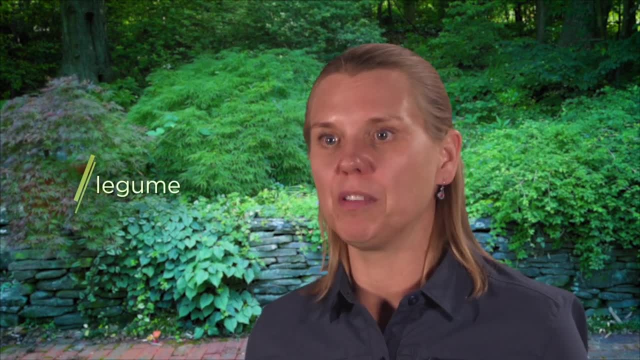 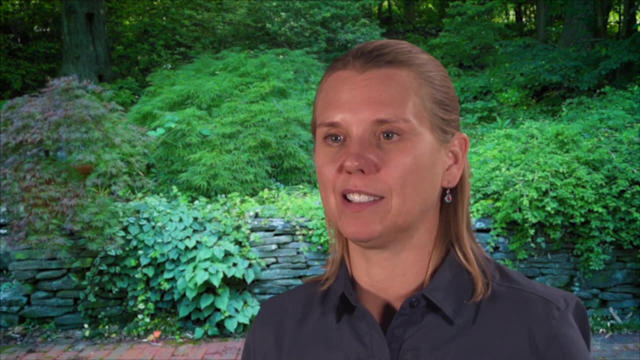 legume and if you're familiar with the garden term legume, you'll know that this term includes beans and peas and peanuts- which aren't actually nuts, but we'll get into that. The legume fruit is derived from one carpal and at maturity. 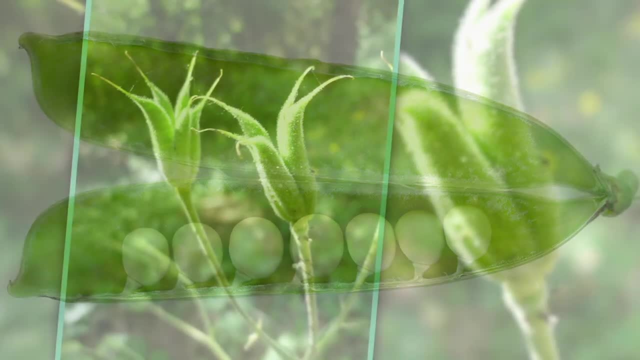 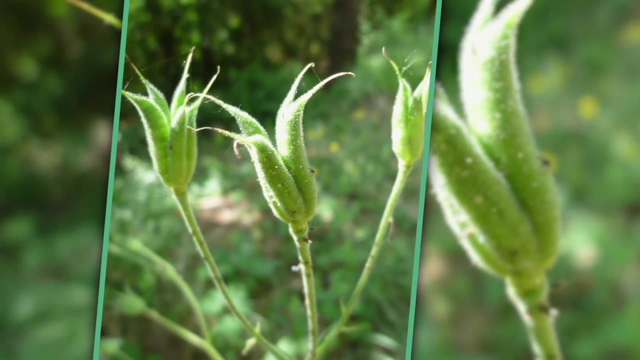 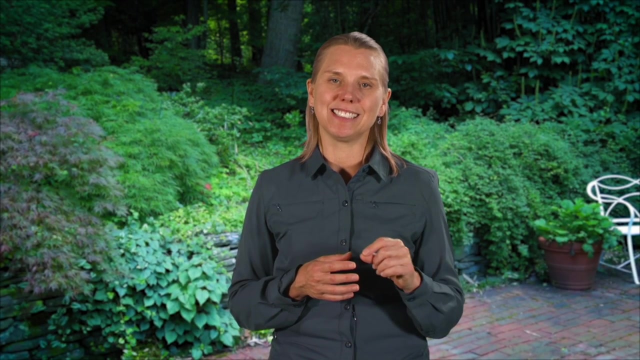 it will split along both the top and the bottom. Similarly, a follicle is a lot like a legume, but it will only split along one side. An example here is the state flower of Colorado, the columbine. Remember we said that the ovary could contain several carpals, or chambers within the ovary. 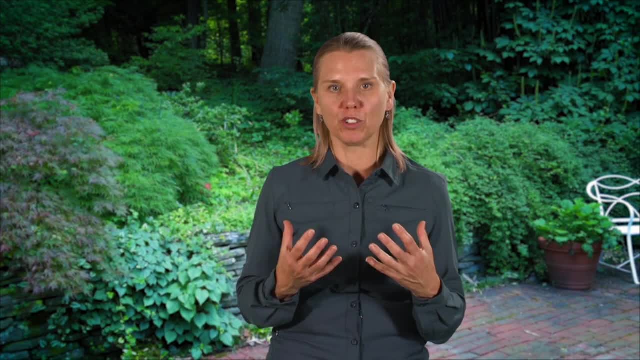 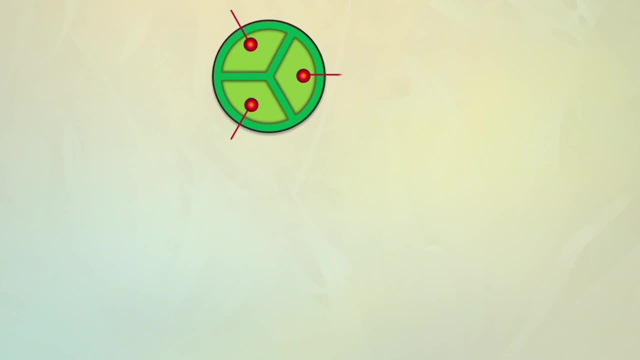 A capsule is derived from several carpals and there are several variations on this theme, depending on how the capsule splits. If the capsule splits in the middle of the locules, then it's called a locucidal capsule, and lilies and irises are good examples. If the capsule splits, 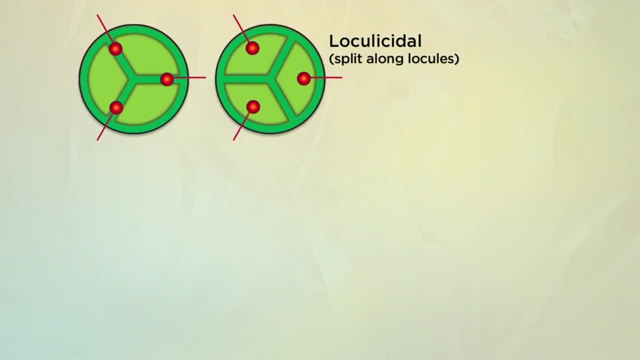 along the wall of the capsule. then it's called a locucidal capsule, and lilies and irises are good examples of the locules which are called septa. then it's called a septicidal capsule And these capsules will open at the top. 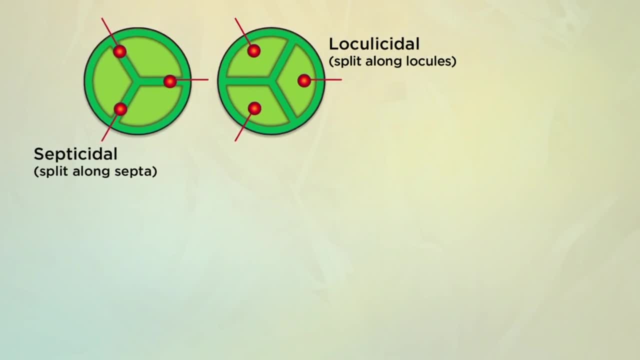 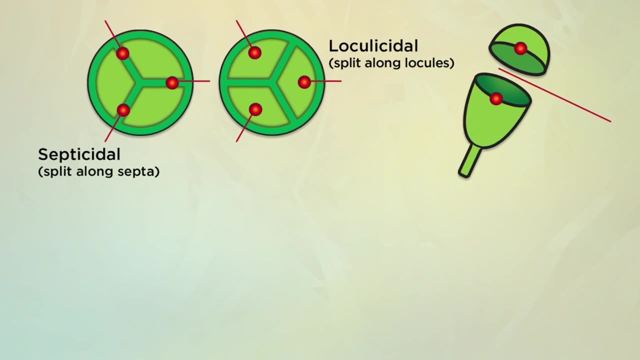 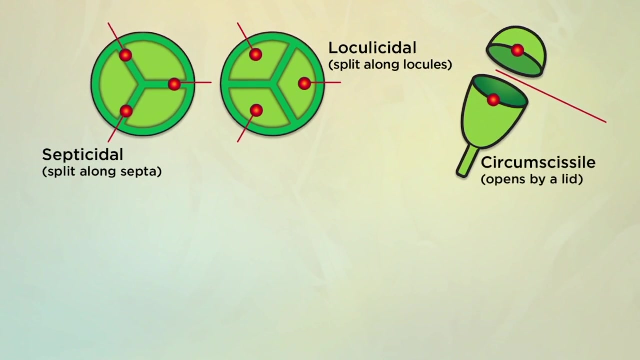 The fruits of yucca and agave provide good examples of septicidal capsules. A pyxis is a capsule that has circumcisal dehiscence, splits along a horizontal line that goes all the way around the fruit or circumscribes it. hence the name circumcessile. 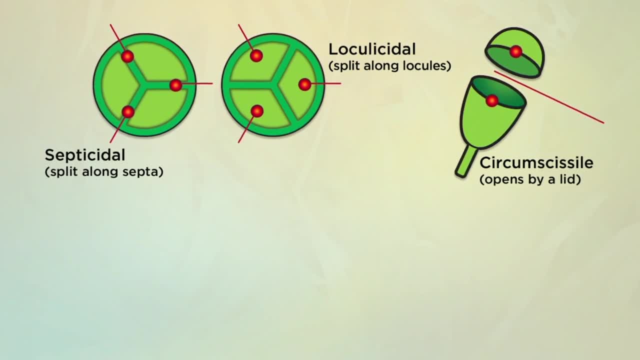 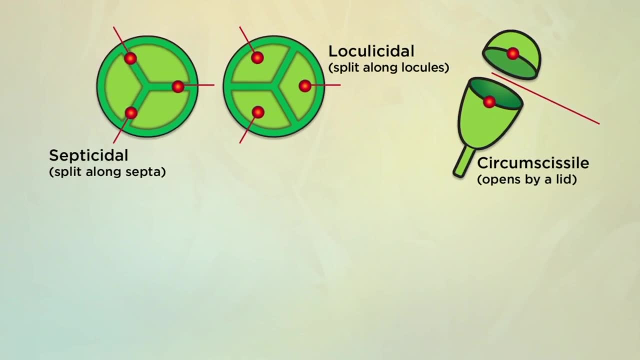 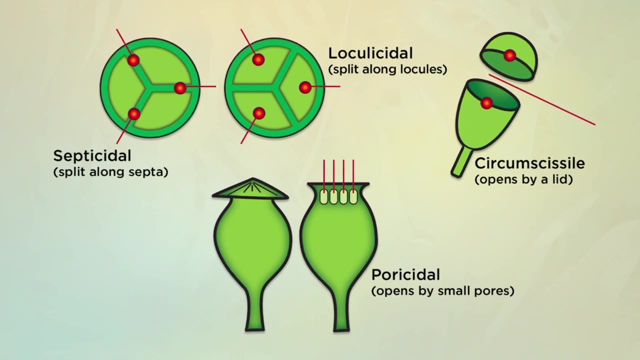 Essentially, this is like the lid of the fruit popping off to release the seeds. Purslane is a good example of a plant with a circumcisile capsule. Perhaps the most ornamental of this group is the poricidal capsule, which will have round holes on the fruit. 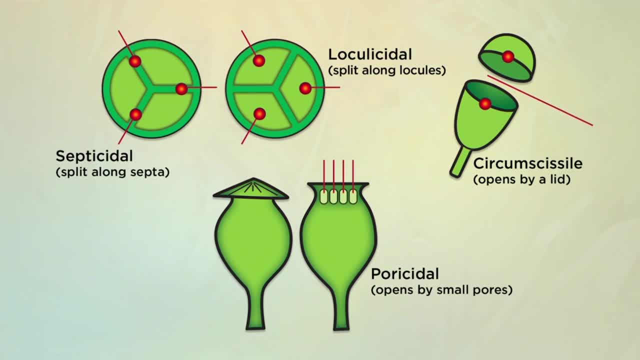 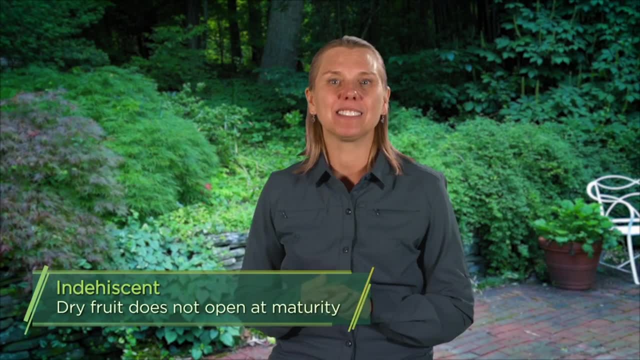 through which the seeds are released. The most famous example of the poricidal capsule is the poppy fruit. Dry fruits can also be indehiscent, which means that they will not open when they mature. You may be wondering how the seeds will be dispersed. 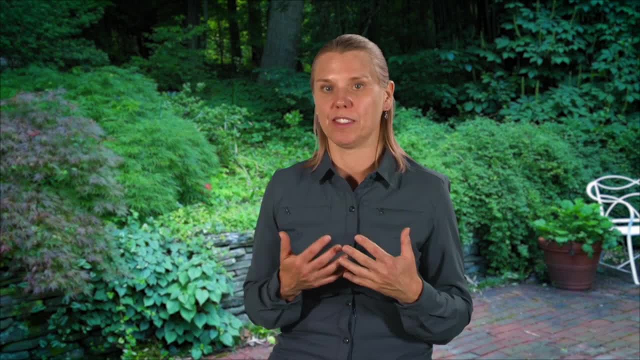 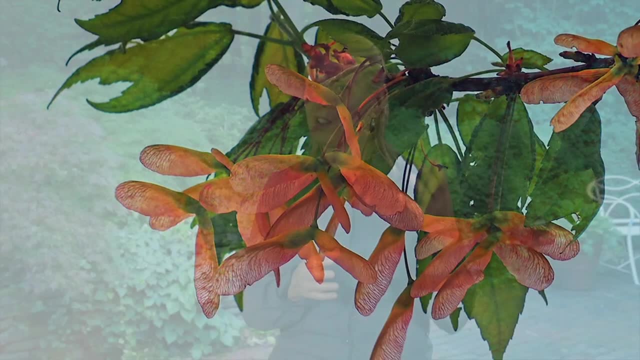 Remember that the fruit itself may be dispersed along with the seeds, and that is the case here. Most of the indehiscent dry fruits are one-seeded fruits. We'll start with everyone's favorite, the whirlybird samara from a maple tree. 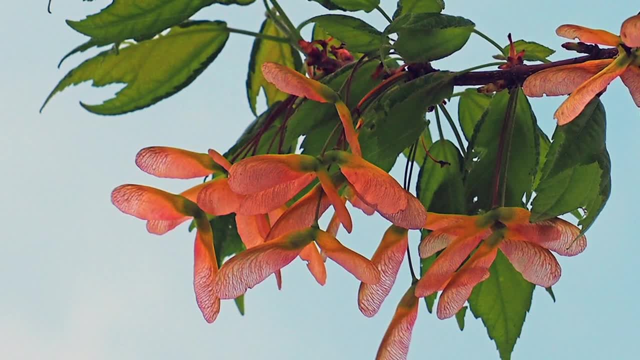 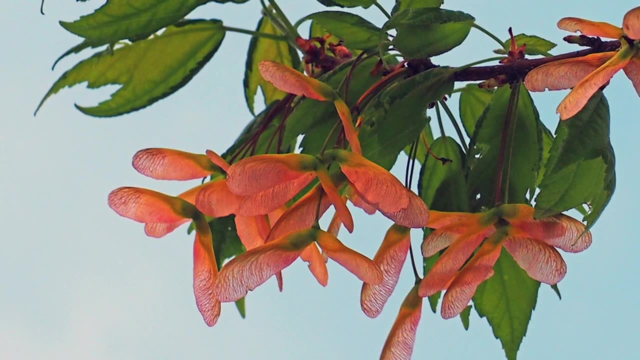 A samara's defining character is that part of the fruit wall grows into a wing. that creates the whirlybird kids love to play with Apparently. the wing aids in secondary dispersal, that is, after the fruit falls initially from the tree. 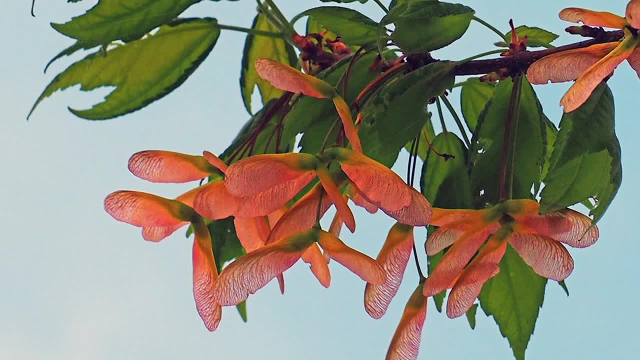 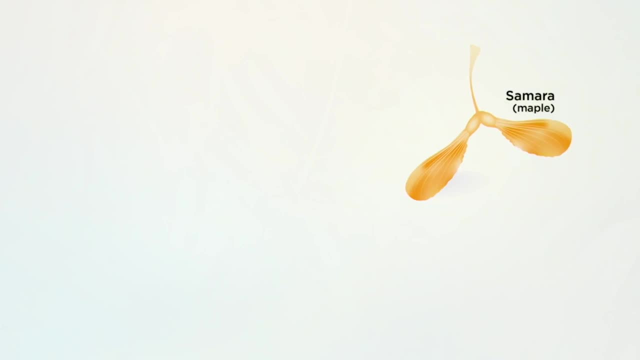 The wing can help it ride the wind a second time away from the parent plant. I think it's good to talk about a schizocarp next, because the double samara can also be defined as a schizocarp. The prefix schizo means split. 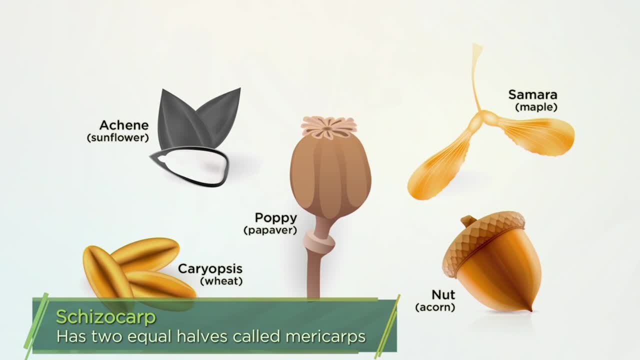 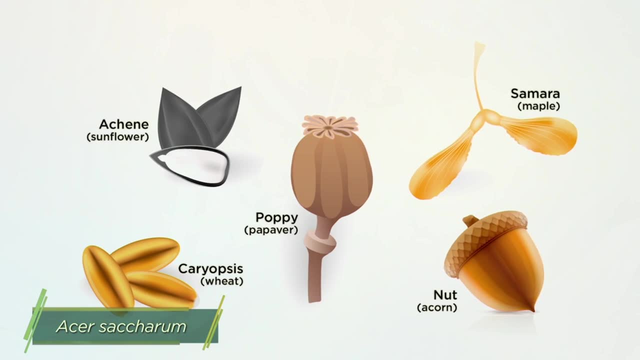 and the schizocarp has two equal halves, each called a mericarp. So when a double samara common to sugar maple or acer saccharum, each samara is a mericarp, So this fruit is a schizocarp. 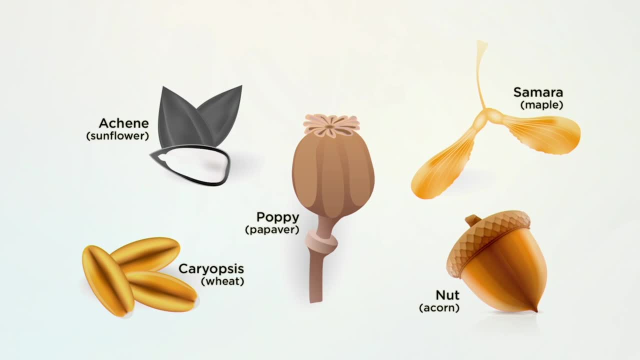 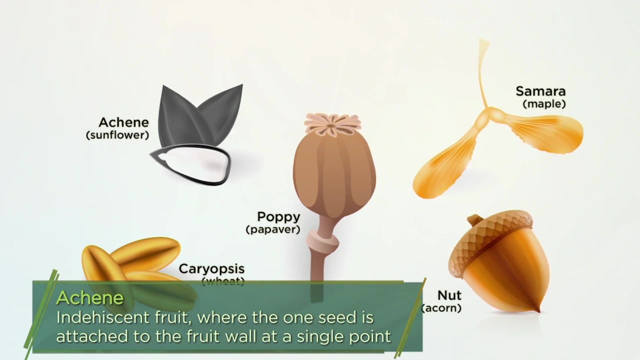 If you've ever eaten a sunflower seed in the shelf, then you've cracked open an achene. This is a one-seeded indehiscent fruit where the one seed- think of your sunflower seed- is attached to the fruit wall at a single point. 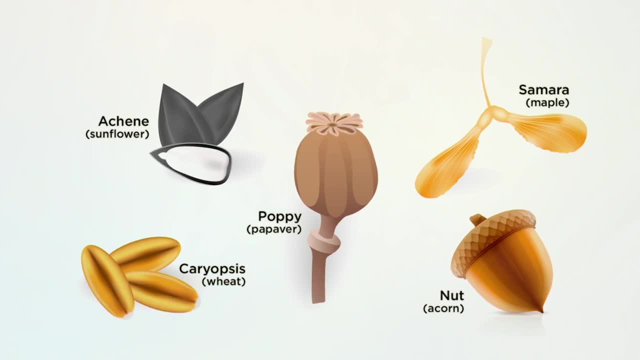 Though it's not apparent in the sunflower seeds in the store, many achenes will have a protrusion, almost like a beak, out of one point of the fruit. Remember I said earlier that a peanut is not a nut, because a peanut is a legume. 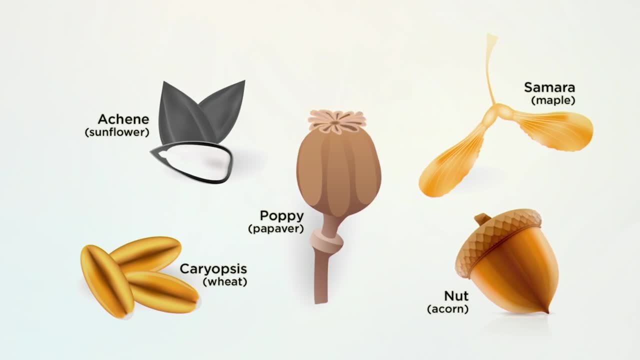 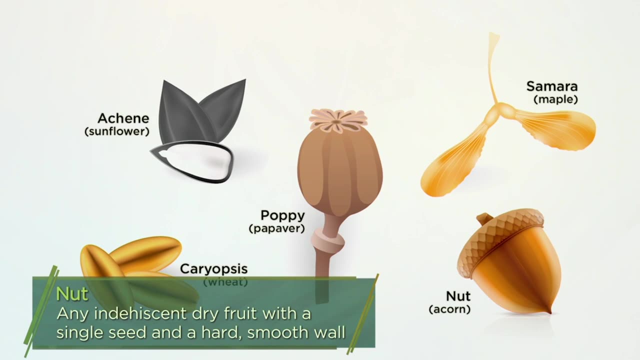 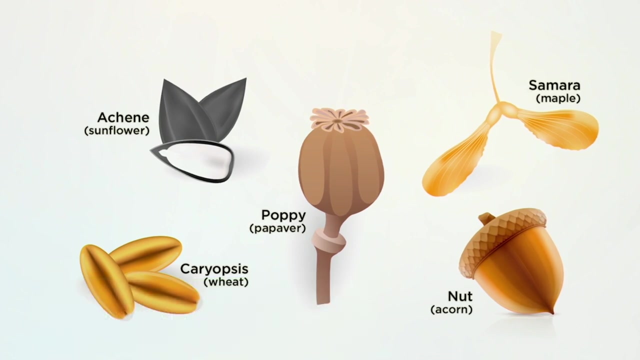 Well, a coconut is not a nut either, and neither is an almond. We'll learn what those are in a minute. In botany, a nut is any indehiscent dry fruit with a single seed and a hard, smooth wall. Also, nuts tend to have caps on them. 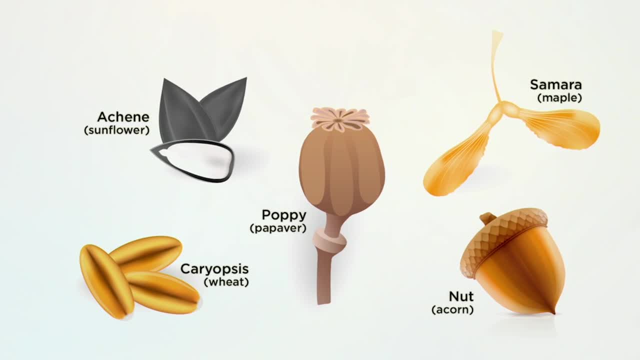 which are really part of the old flour that fuses together. This is true of an acorn, which is a nut. It's hard-walled and has a cap or a cup on it. Our last indehiscent dry fruit is grain or a karyopsis. 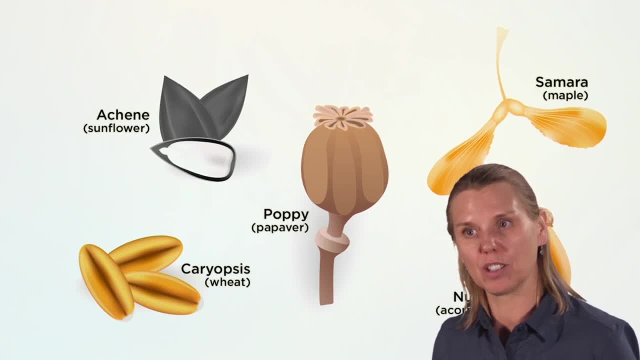 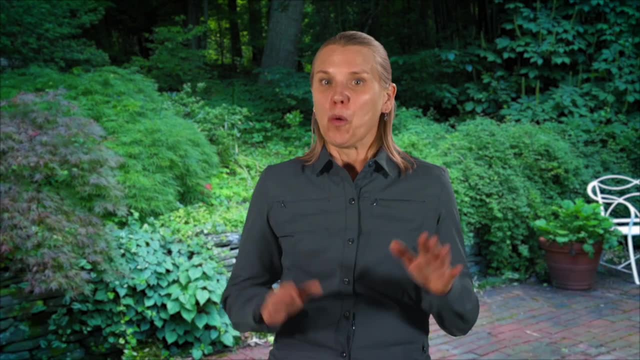 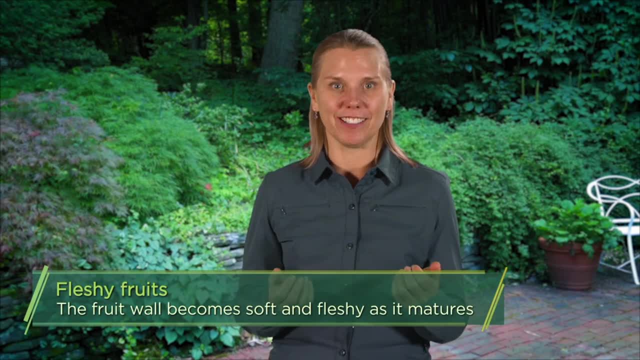 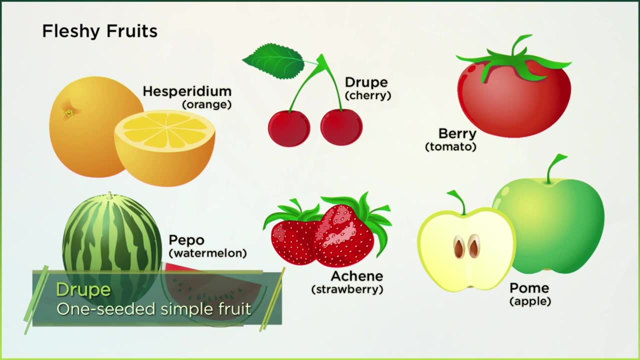 we'll move on now to fleshy fruits where, just like it sounds, the fruit wall becomes soft and fleshy as it matures. A drupe is the fruit type for some of our most beloved fruits. Drupes are one-seeded, simple fruits. 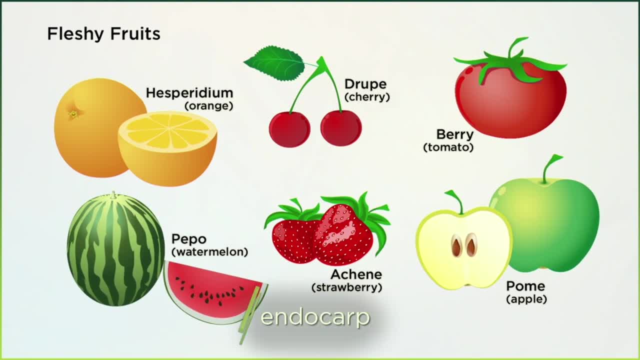 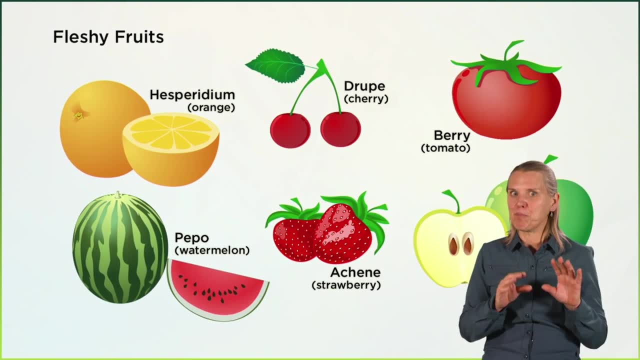 The innermost portion of the fruit wall, which is called the endocarp, becomes hard and stony, and this is the part we call the pit. So think of peaches, plums and cherries: They all have pits. 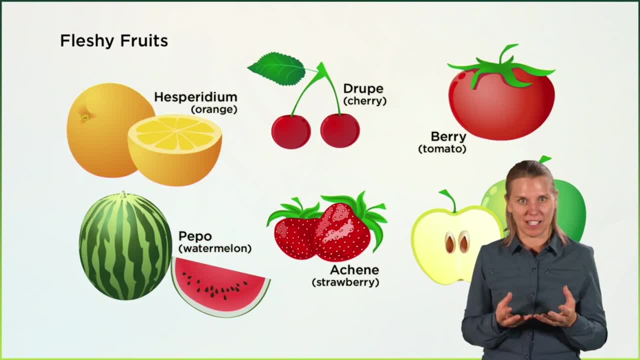 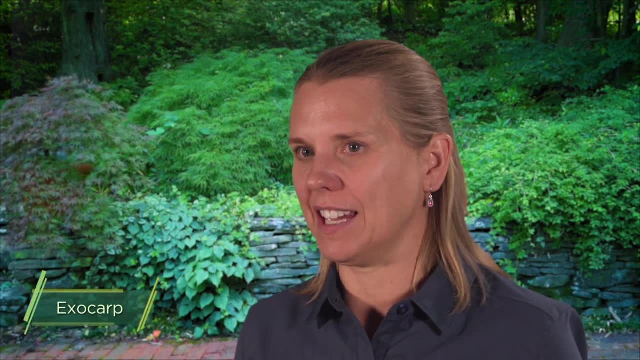 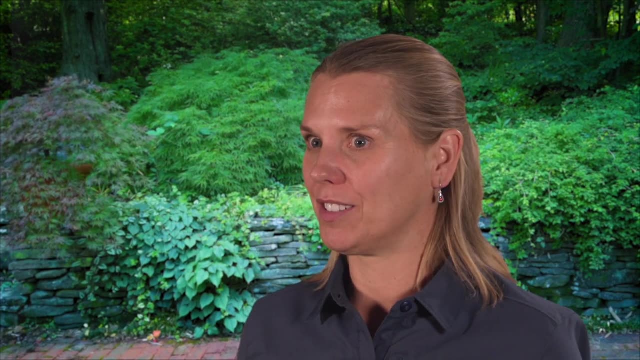 So a pit is a hard is a hard covering around the seed. The outermost part of the fruit, called the exocarp, becomes a relatively thin skin and the middle portion between the skin and the pit becomes either fleshy or fibrous. 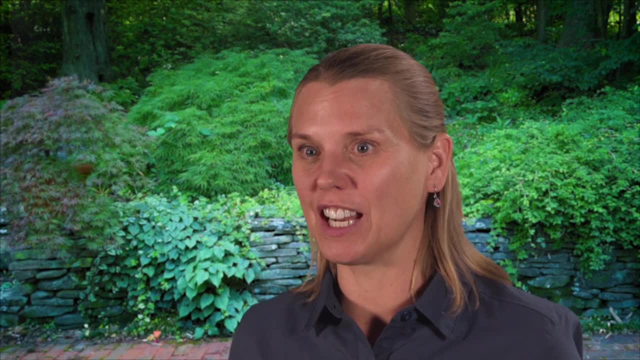 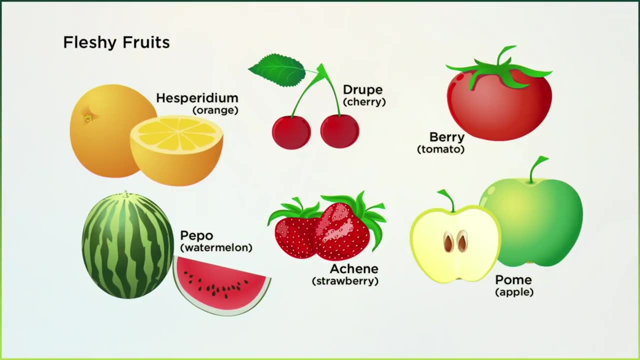 What about a coconut? If you've ever seen a fresh coconut, you know that it comes in a large fibrous husk. so it's also a drupe If the fleshy fruit has a seed that is not enclosed in a hard covering. 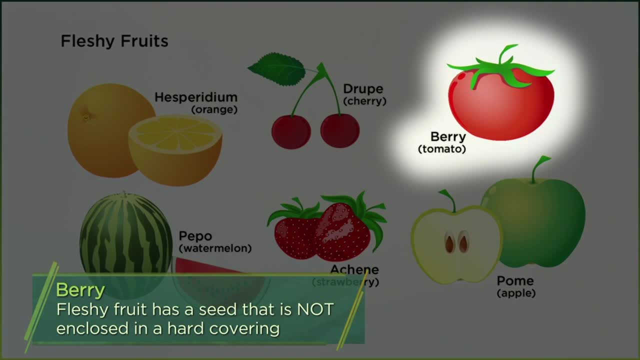 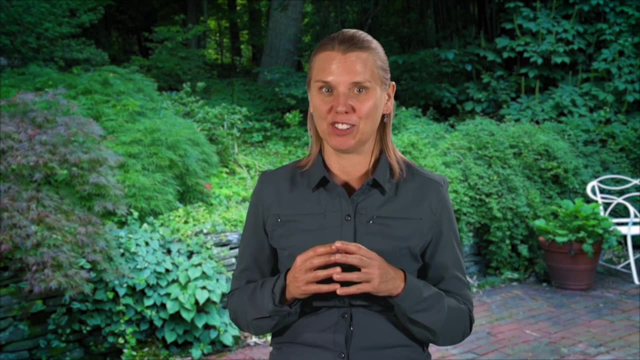 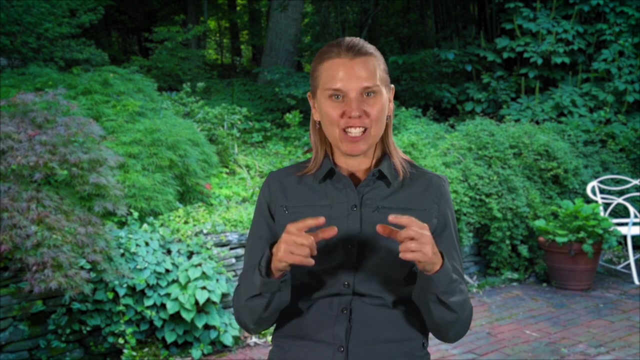 then it's a berry. This includes almost all fruits with more than one seed, like tomatoes and grapes. Here's some real botany trivia too. What about an avocado? It seems to have a pit, but the hard thing in the middle is really the seed. 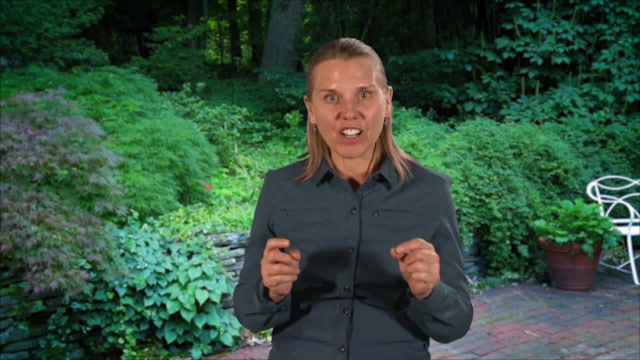 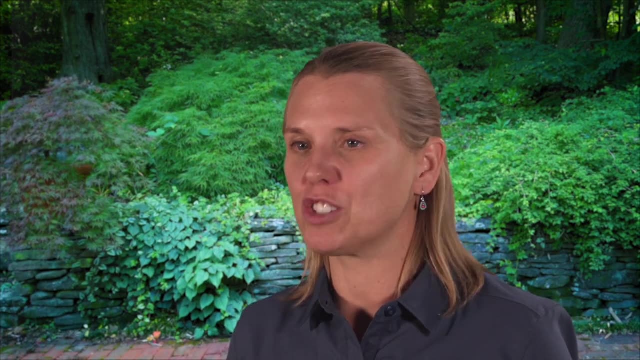 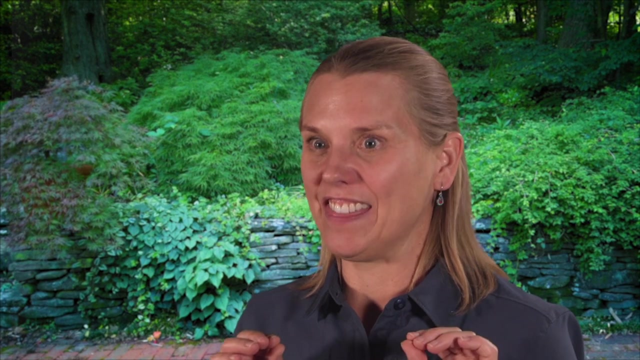 not a hard covering around the seed. So an avocado is a berry. There are two special types of berry-like fruits that I like to mention solely for the fun of saying their names in the grocery store. The first is a berry with a leathery rind. 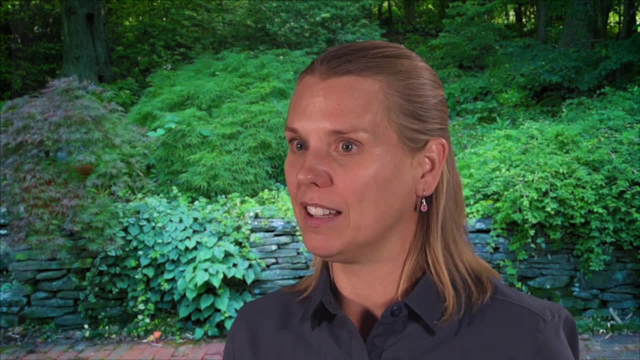 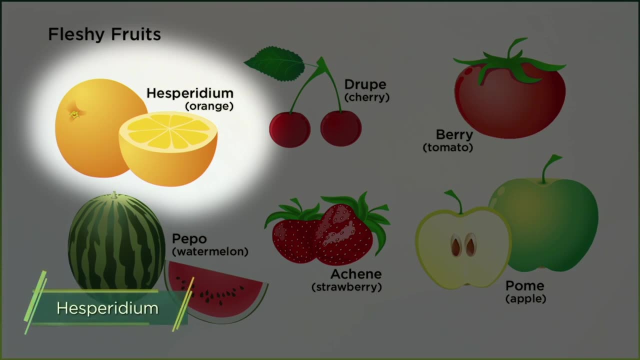 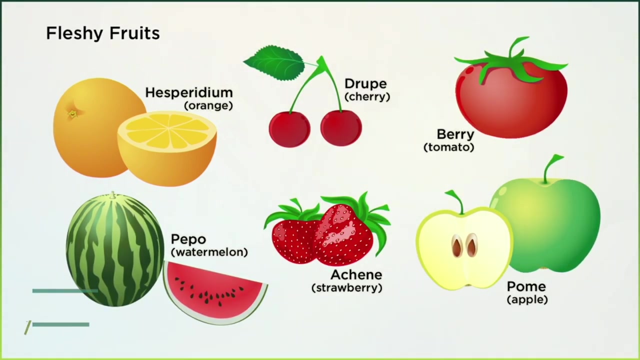 and the interior of the fruit is divided along septa into the carpels. Think of an orange. This is a special berry called a hesperidium. Now think of that same berry, only with a hard rind, and you have a pit. 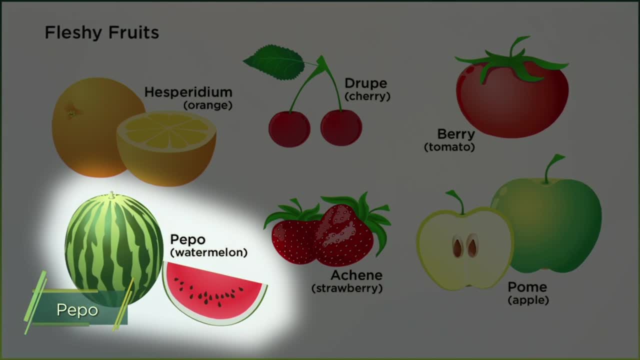 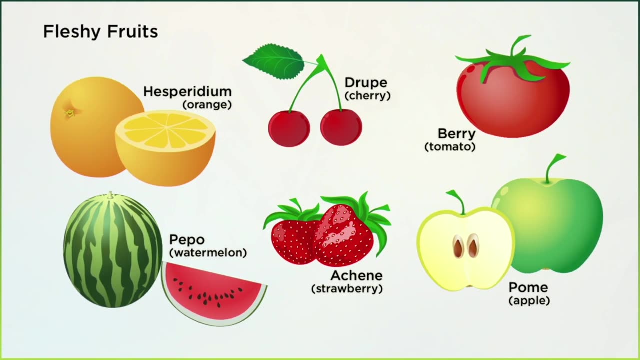 This is a peepo, which would be a watermelon or a squash. Our last fleshy, simple fruit is a pomme, and if you know French, you'll already guess that this is the fruit type for an apple. A pomme is actually an accessory fruit. 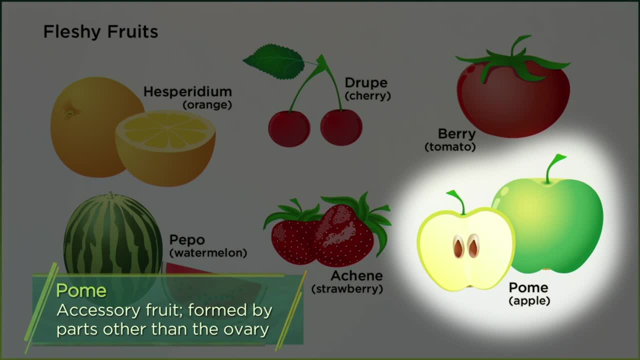 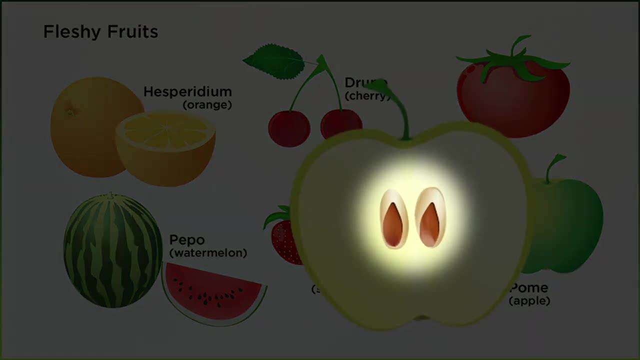 which means it's formed by parts other than the ovary. Where is the ovary in an apple? It's in the very core and if you slice the apple just right, you can see the papery, the outer layer around the ovary. 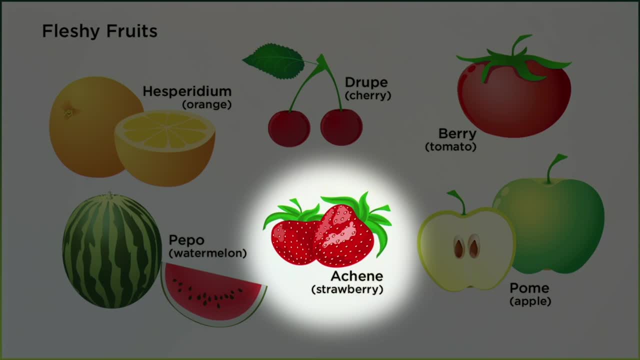 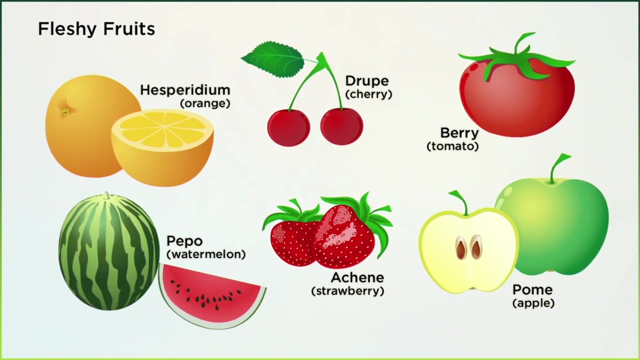 Another accessory fruit is strawberry, which isn't a berry at all. Why not? There aren't multiple seeds inside, surrounded by a fleshy fruit. No, in a strawberry the seeds are on the outside, though they are not actually seeds.